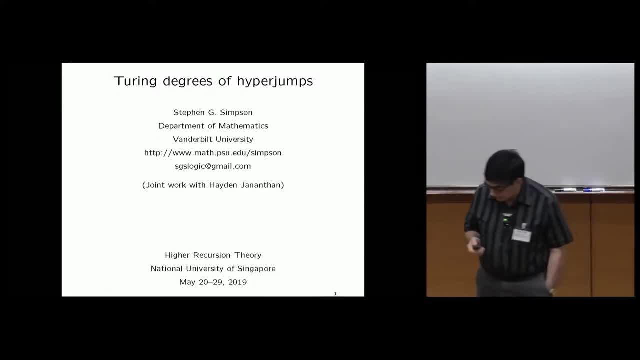 So maybe you're wondering why I'm at Vanderbilt University but my website is. My website is at PSU, which is Pennsylvania State University. That's because I'm affiliated with both universities. I retired from Penn State some years ago and, with my wife, moved to Vanderbilt University. 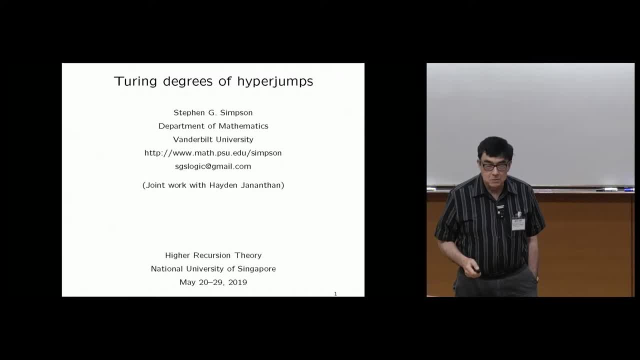 It's a Well, we like to call it the Harvard of the South. It's in the southern United States, but it has the atmosphere of an Ivy League school. I must say It's a private university and it has that feeling and it's a very good university. 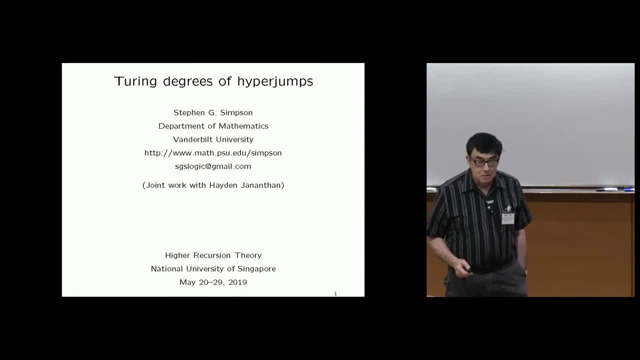 And my title there is research professor, which is I don't get a salary but I'm treated as a professor. I can work with students and so on and apply for research grants, things like that. So that's where I am. 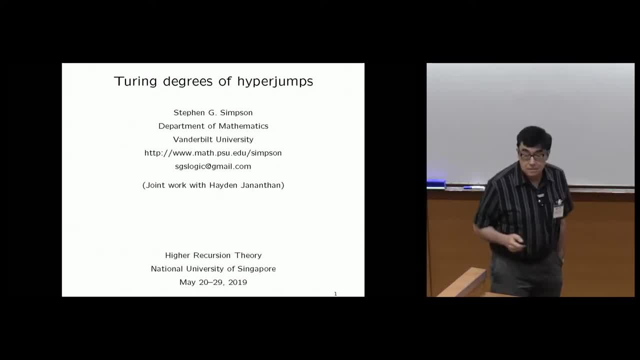 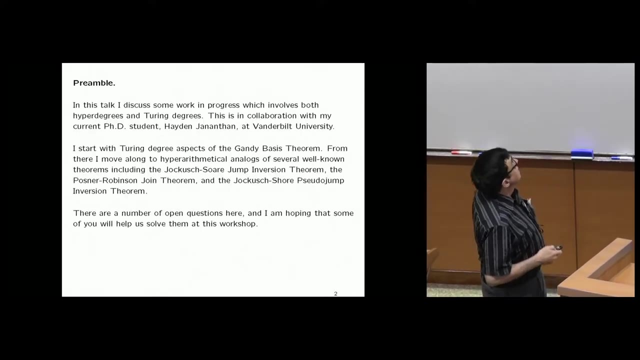 This is In the talk. I'll be discussing some current work in higher recursion theory with Hayden Jananthan. He is Well. let me go to the next slide here. He is a PhD student at Vanderbilt University and he's just getting started. 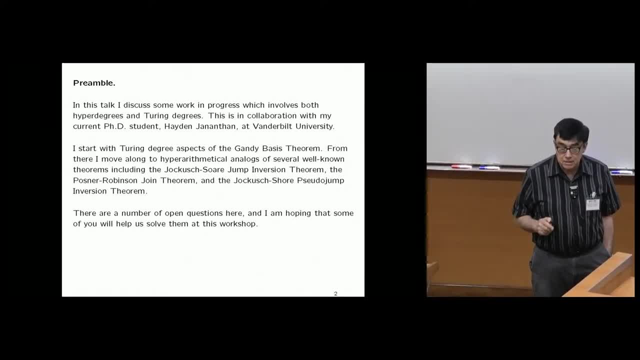 I mean, he's very good and very energetic, but I don't know if I don't know whether his PhD thesis will be about recursion theory directly or not. but I mean, you know he's interested in many things, but this is some work that we've 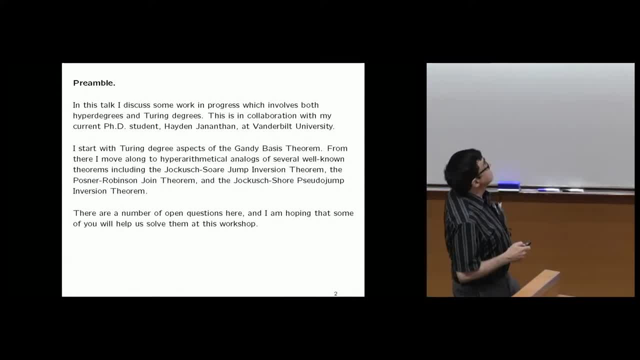 been doing just recently And let me say about this, this is work in progress. very much. I was encouraged by the fact that this meeting here is called a workshop, not a. I don't know if you've heard of it, but it's called a workshop. 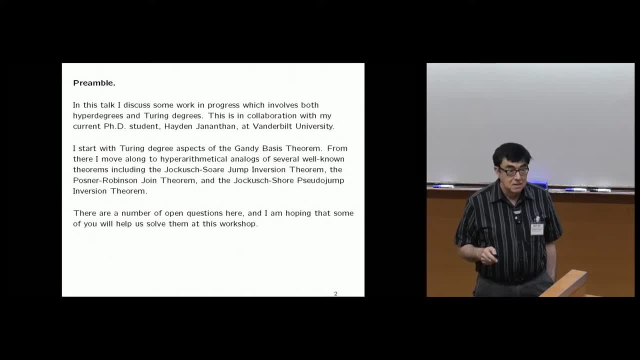 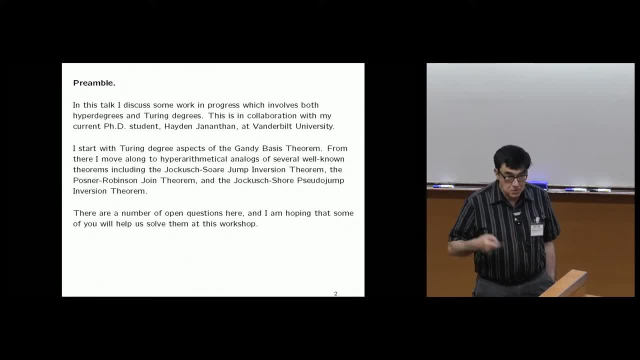 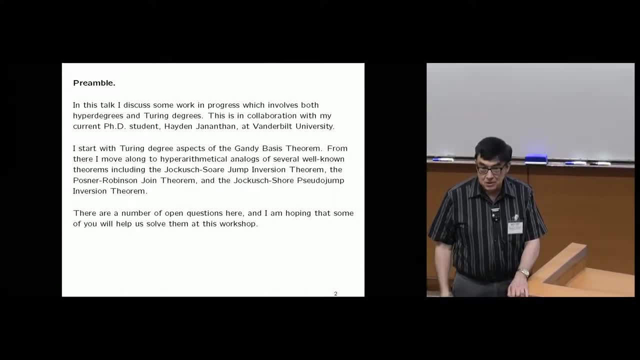 work in progress and I hope all of you will help me to solve the open problems that I mentioned. There are many open problems here, at least I don't know the answers to and I don't know, I don't know. 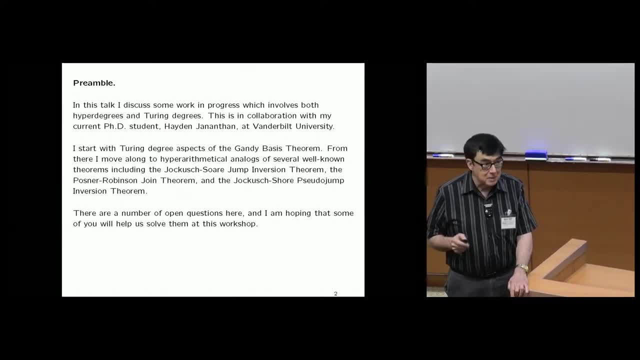 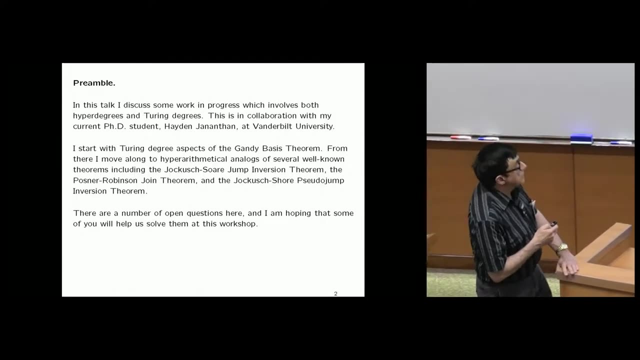 I don't know. Some progress has already been made at this meeting or as a result of this meeting here, this workshop, and I'll tell you about that during the talk. The slides were prepared before I came here, So I'm going to spend a good deal of time. 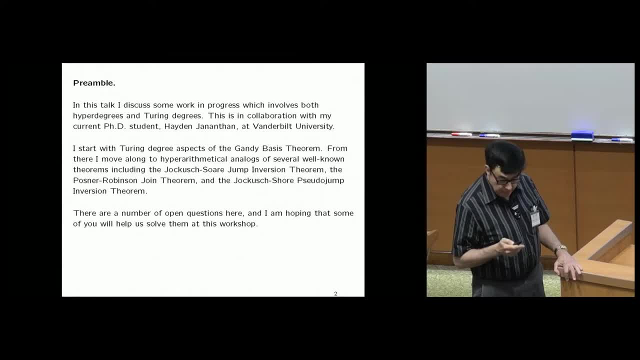 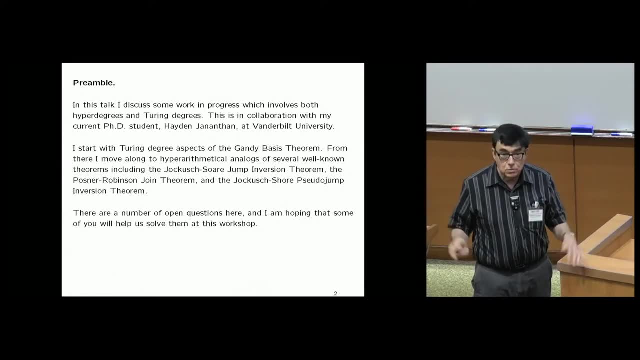 talking about theorems related to the Gandhi basis theorem. Antonio has not in his. He's giving a tutorial on hyperarithmetic theory and structure theory. He mentioned some aspects of this already, but I'll Well, I don't know how it. 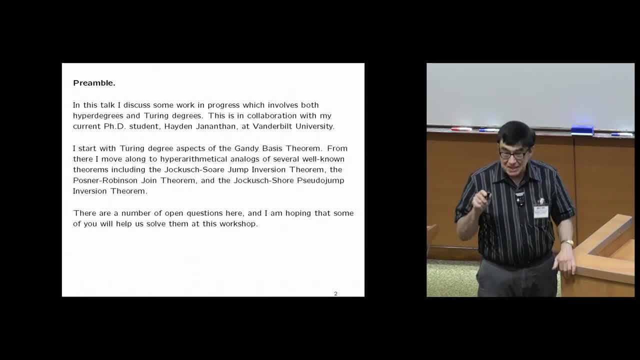 It's very. That's another reason that I decided to talk on this. I decided to talk on this topic at this meeting because there's obviously a lot of interest here in hyperarithmetic theory, with Antonio's tutorial going on- Okay. so hyperarithmetic theory, let me say. 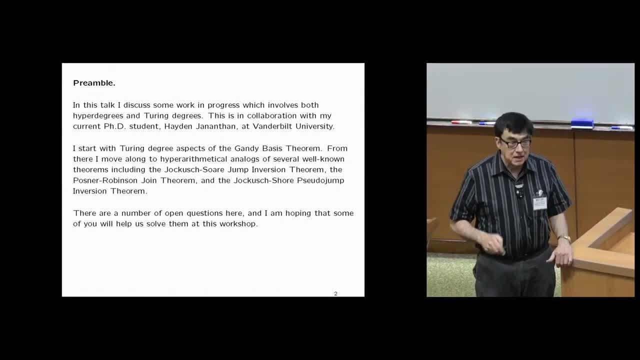 is chapter one or part one of higher recursion theory. There's more to it And one of the There's the book of my And Ted's thesis advisor and Gerald Sachs called Higher Recursion Theory, And part A of the book is hyperarithmetic theory. 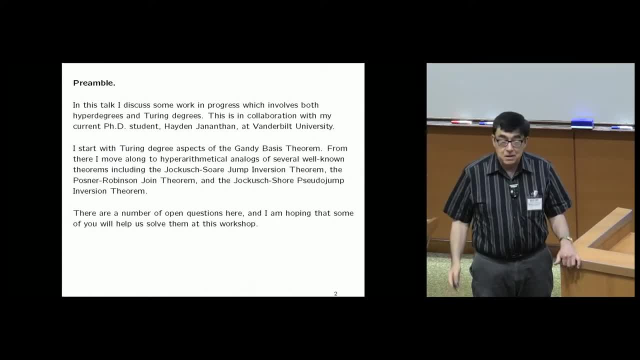 And then the later parts have to do with other kinds of hyper, Other kinds of higher recursion theory, alpha recursion theory and E recursion theory and so on and so on. There's a lot of you know, interaction with between recursion theory and set theory there. 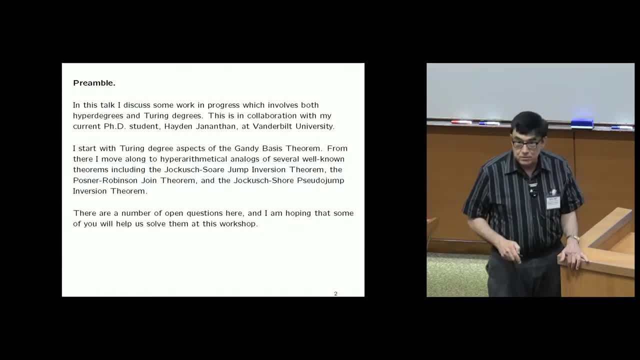 But this is just a very basic part of higher recursion theory, Historically the first part. So okay, Okay, Absolutely, I've done. I think somebody in a different life I think I did that, Okay, Okay, right. 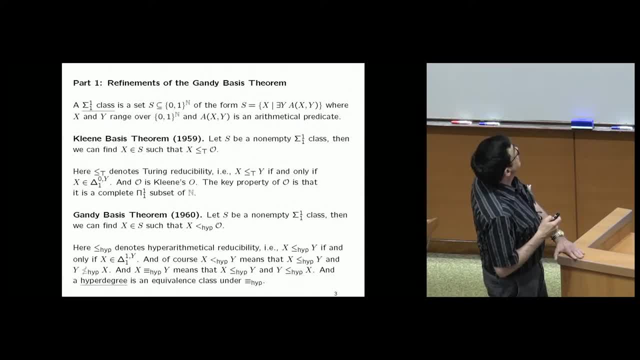 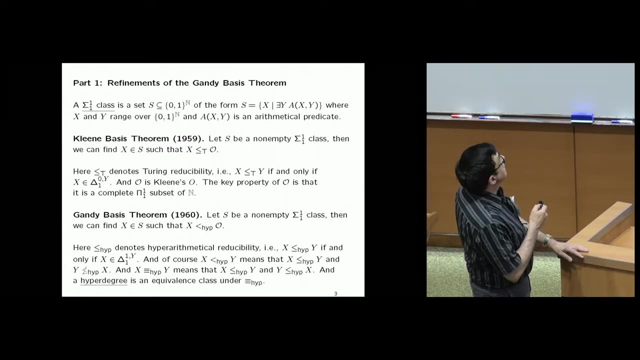 So. so let's see. I want to first want to state the Gandy basis theorem: A sigma one one class is a, So zero one to the n is the is the Cantor space, And a sigma one one class is a set. 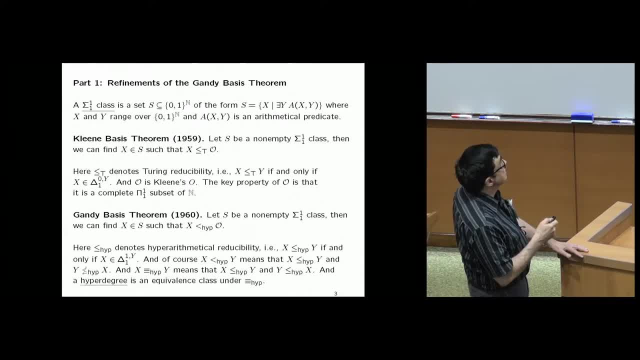 a subset of the Cantor space, which is sigma one, one which means that it's it's of this form, an arithmetical predicate preceded by an existential problem. It's an existential quantifier over points in the Cantor space. 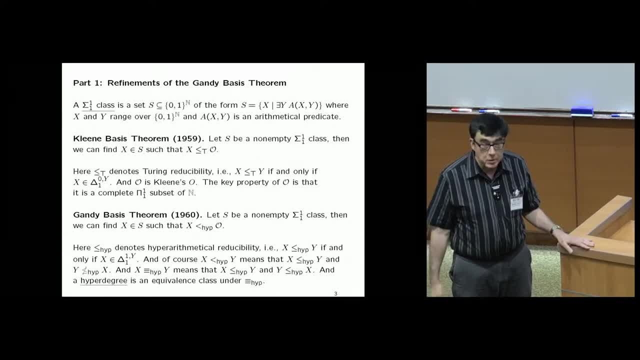 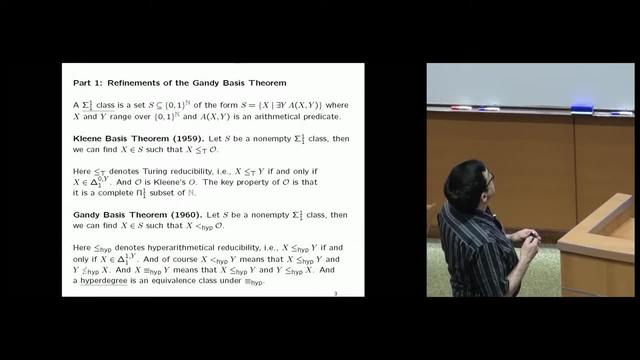 which I may call reals. You know everybody calls them reals in this field- Just points in the Cantor space. So I hope this is clear. It's not important here that S should be a subset of the Cantor space. 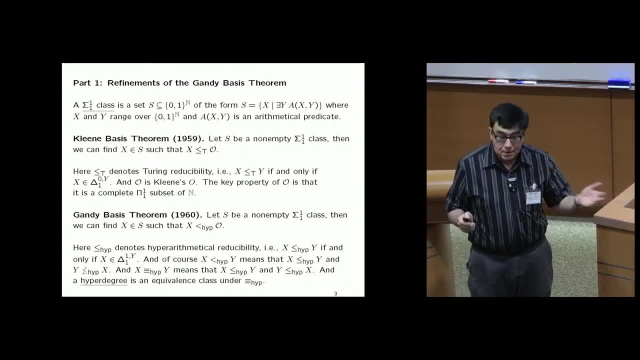 It could equally well be a subset of the bare space, But later I'm also going to talk about pi zero one classes, where it is important, That's. that's an important distinction, You know, the point being that the Cantor space is compact. 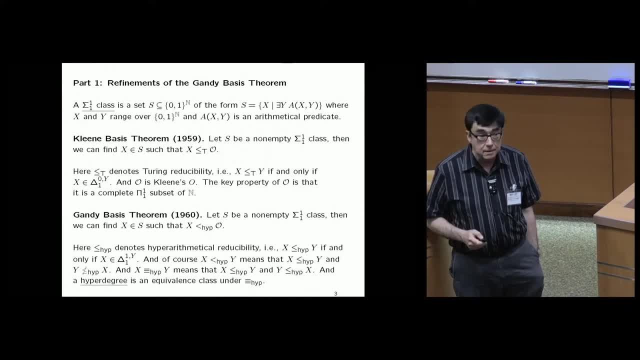 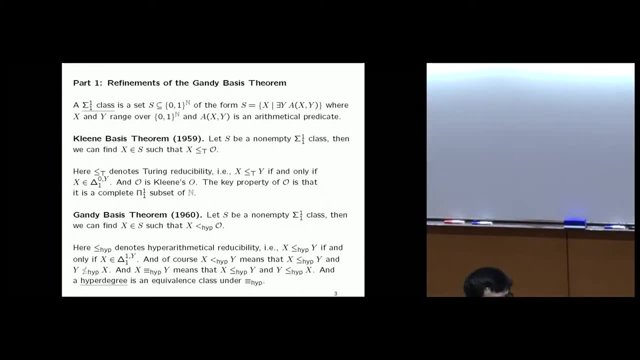 while the bare space is very far from being compact. Okay, so the Kleene basis theorem? I've seen this. I mean, Gerald Sachs used to call this the Kleene basis theorem. I think it's called that, but I wasn't quite able to track down the reference. 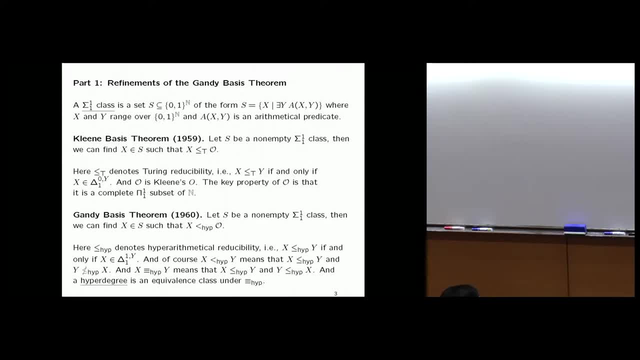 But it's here's what it says. Let S be a nonempty sigma, one, one class. Then it has an element which is Turing reducible to Kleene's O. Antonio has already explained Kleene's O. It's well as I'll explain. it's the 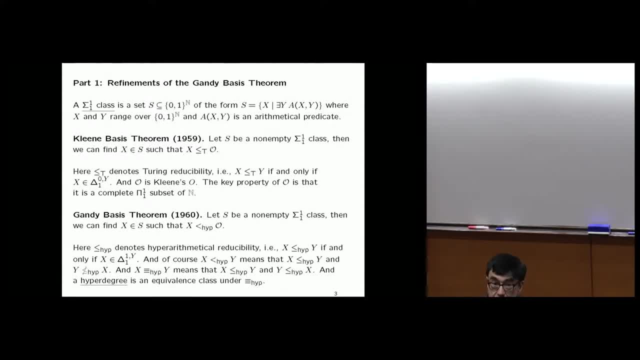 it's the analog of the halting problem in recursion theory. Basically, there's recursion theory. where you're dealing with. the beginning of that subject is the unsolvability of the halting problem. And then you move to hyper arithmetic theory and the beginning of that subject is the fact that 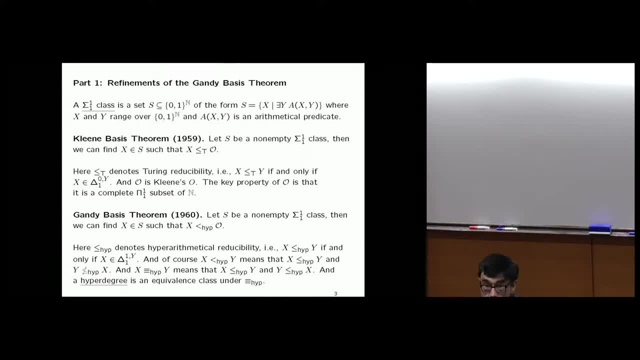 Kleene's O is not hyper arithmetical, but it is pi one, one And so, and it's, and there's a strong analogy, which I want to emphasize, between recursion theory and hyper arithmetical theory. So let's see, just explaining all the terminology. 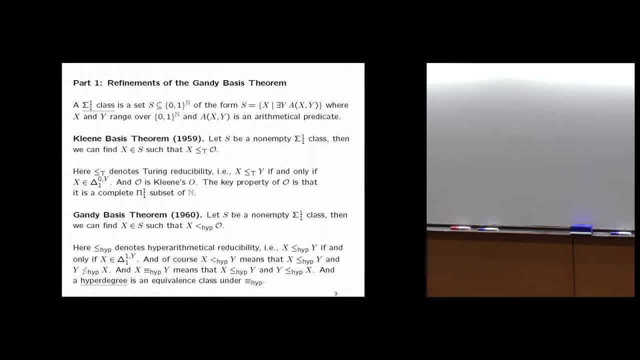 Less than or equal sub T. you know it's Turing reducibility, That is, X and Y being points in the Cantor space. X is Turing reducible to Y if, and only if, X is delta zero one in Y. 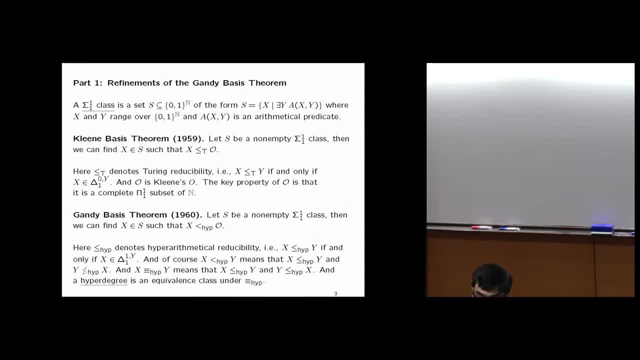 Or another way to say this, is that X as a function, as an infinite sequence of zero ones, that sequence is computable using the infinite sequence of zeros and ones, Y as a Turing oracle, In other words, you're allowed to call on 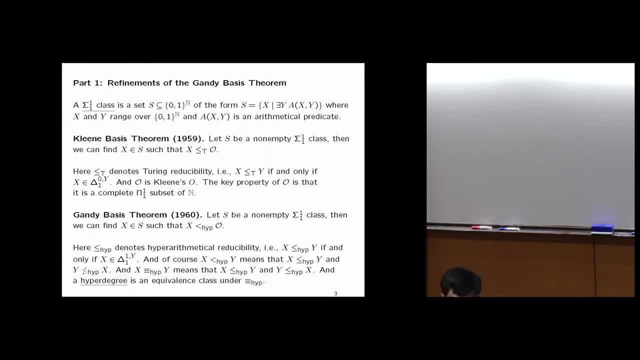 finite pieces of information about Y as you go along. So that's Turing reducibility, And so so we're going to do, we're going to deal more with Turing reducibility, but I'm also dealing with hyper arithmetical reducibility in this talk. 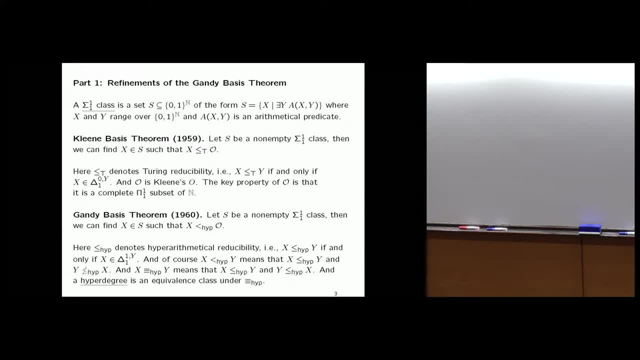 But an O script O is Kleene's, what Kleene called just capital O O, And the key property of it is that it's a complete pi one, one subset of the natural numbers. Antonio explained all this in his tutorial and maybe, maybe I want to assume that that makes sense to everybody. 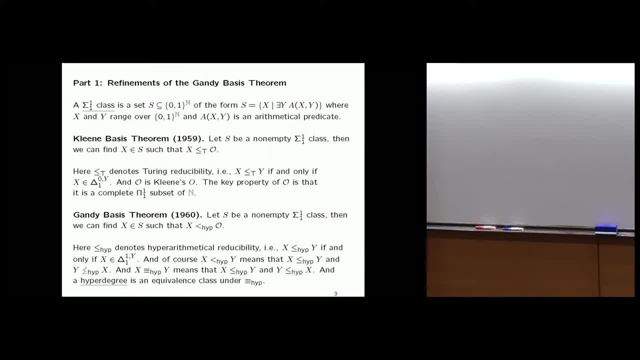 Well, the and this is this- is just like the halt, it's, it's the analog of the halting problem. I mean, O is a complete pi one, one set of natural numbers, just like the halting set is a complete, recursively enumerable subset of the integers. 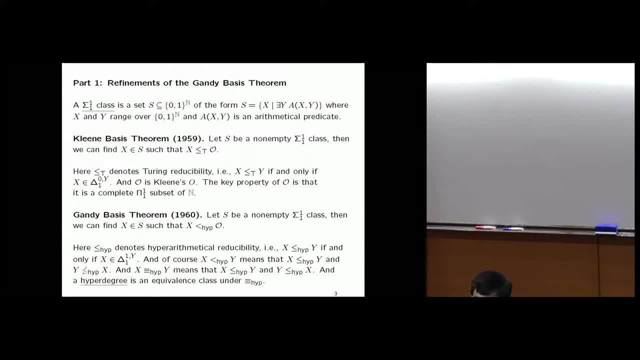 And in fact pi one one sets are analogous to recursively enumerable sets or sigma zero one sets, And so that's the analogy, All right. so anyway, this is the Kleene basis theorem, and there's an analogous theorem for pi zero one classes. 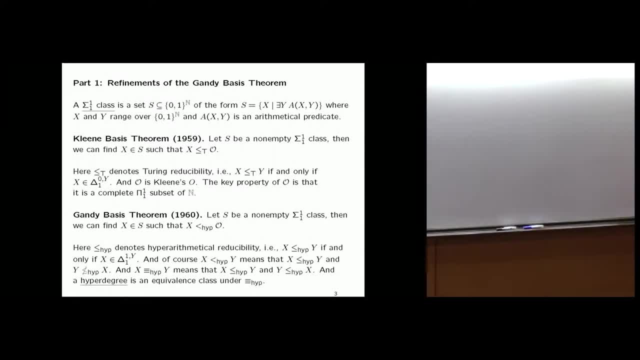 Of course there's an which is also called, I believe, the Kleene basis theorem, And in fact the two theorems are stated together in one theorem. They're just, they're variants of each other. Okay, So this is very old stuff. 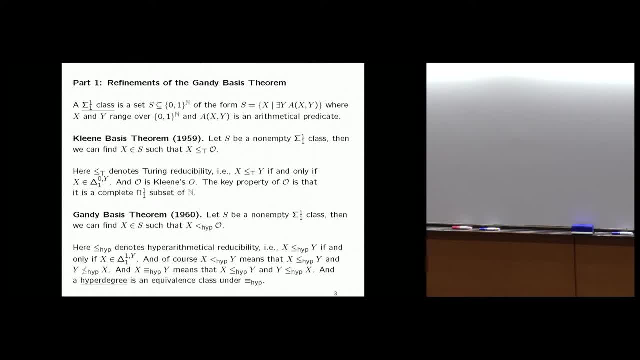 The Gandhi basis theorem is a refinement. Well, it's not exactly a refinement. Here's the way Gandhi stated it. I actually looked up Gandhi's paper. Here's how he states it. Let S be a nonempty sigma. one, one class. 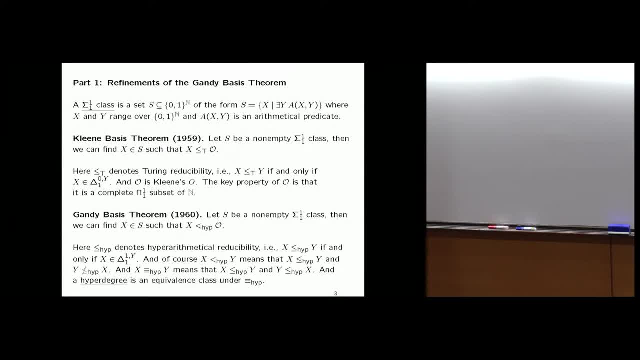 Then we can find a member of S, a point in S which is of strictly lower hyperdegree than O. So I'm not going to say very much about hyperarithmetical reduces. but here are the definitions: Less than or equal subhype. you know it's hyperarithmetical reducibility. 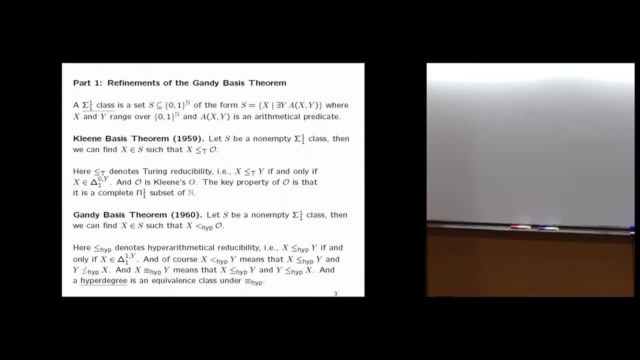 X is said to be hype in Y. if X is delta one one in Y, Delta one one in Y. well, X is hyperarithmetical if, and only if, it's delta one one. X is hyperarithmetical in Y if, and only if, it's delta one one relative to Y. 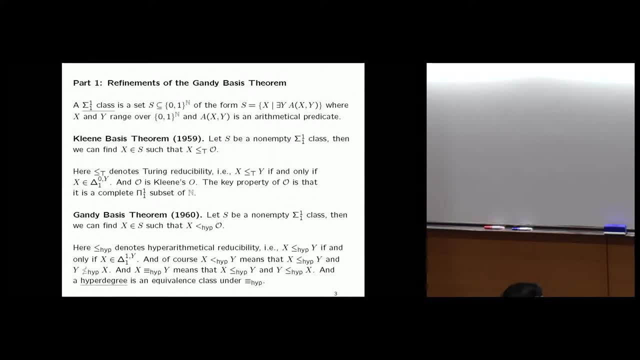 So that's the analog of Turing reducibility here. And of course then less than subhype means less than or equal, but not greater than or equal. And hyperarithmetical equivalence just means that X and Y are each hyperarithmetical in the other. 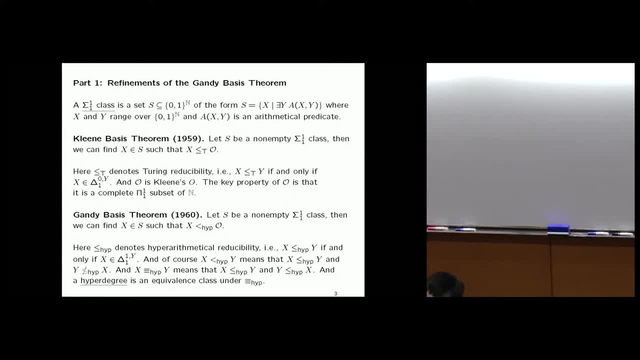 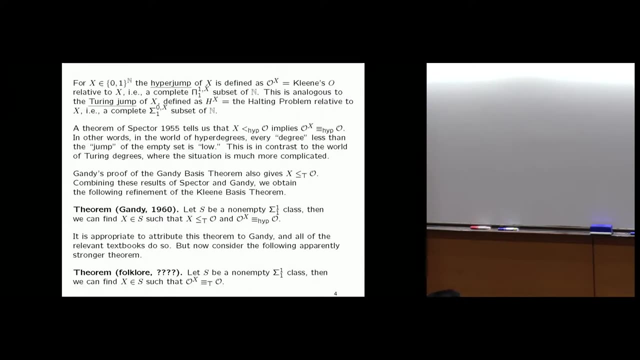 A hyperdegree is an equivalence class under that equivalence relation, just like a Turing degree is an equivalence class under Turing reducibility. Okay, so he's got. so here's this theorem. Now, these theorems are different actually, but you can combine them in this theorem of Gandy here. 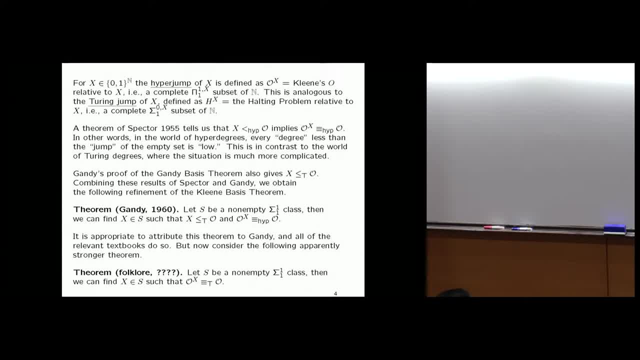 You can say, you can say more, So let me well. so first I have to talk about the hyperjump Given, and this is, and this the hyperjump is going to be mentioned frequently in this talk, more frequently than hyperarithmetical reducibility. 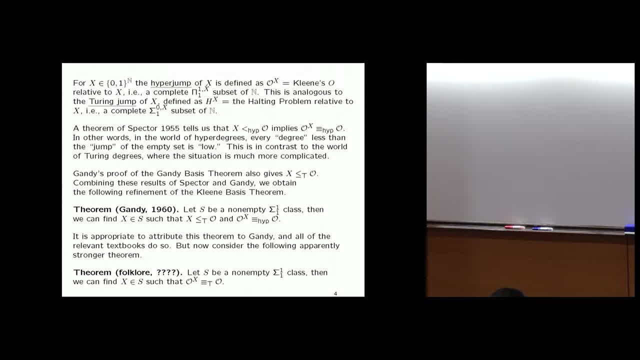 I'm going to mix the two. In other words, I'm going to be talking about hyperjump, but Turing degrees, Turing degrees of hyperjumps- that's the title of the talk. Okay, so the hyperjump of X is O relative to X. 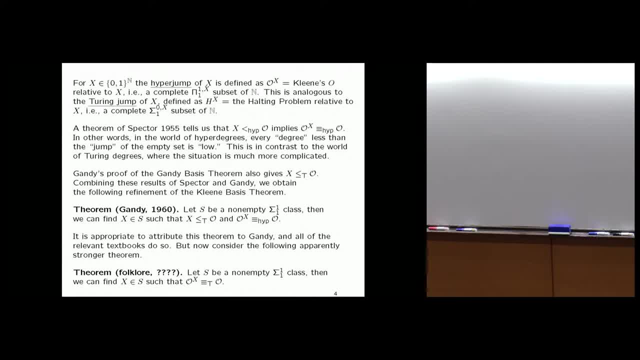 Kleene's O relative to X. In other words, it's a complete pi one, one relative to X subset of the natural numbers. So this is analogous to the Turing jump of X, defined as H super X equals the halting problem relative to X. 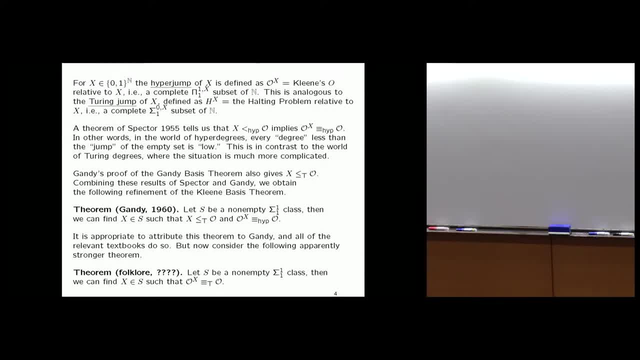 which is a complete. the key property of that for us is that it's a complete sigma zero one relative to X subset of N. So this is, it's analogous. It may look a little strange that sigma zero one is analogous to pi one one. 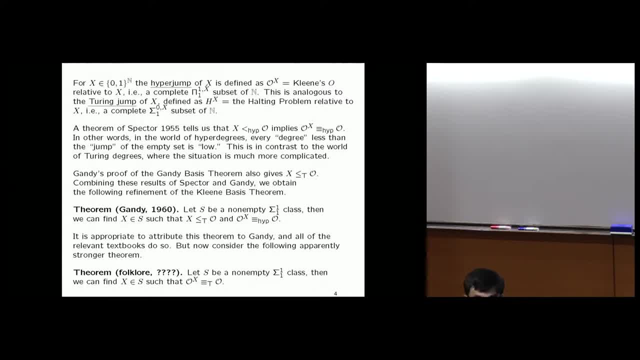 but, believe me, this is the right analogy. If you you have to you you this is. this is a far-reaching analogy. Roughly speaking, stages of computation in recursion theory just correspond to stages of computation, but stages of computation in hyper-arithmetic theory 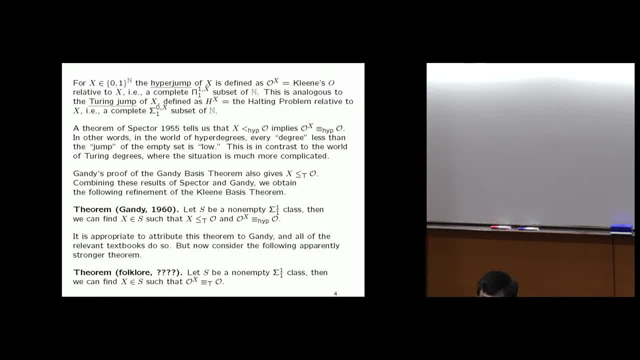 correspond to recursive ordinal. recursive ordinals. That's the idea. All right, Now another theorem of specter. a theorem of specter actually earlier than Gandhi's is that if X is hype in is of strictly lower hyper-degree than O. 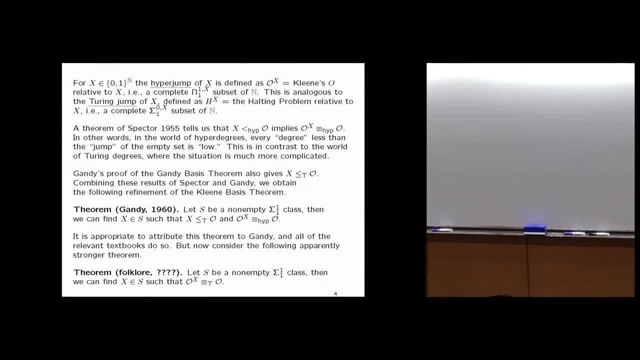 then the hyper-jump of X is hyper-arithmetically equivalent to O. So that's a theorem of that is that's a theorem of specter, quite early before Gandhi, And so Gandhi doesn't cite that, but in his paper. but specter's theorem tells you something very strange. 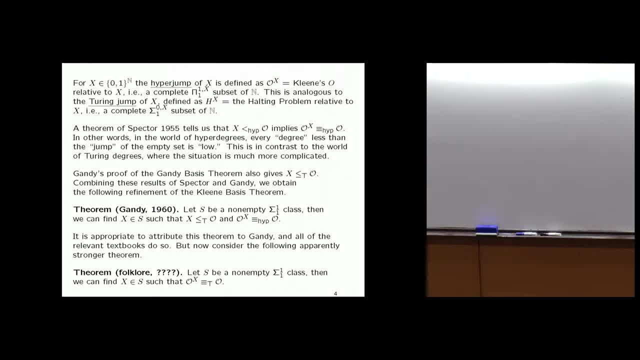 if you're, if you're, a recursion theorist, it tells you that in the world of the see, in the world of Turing degrees, there are degrees that are less than the halting problem, less than zero prime, but their jump is not the halting problem. 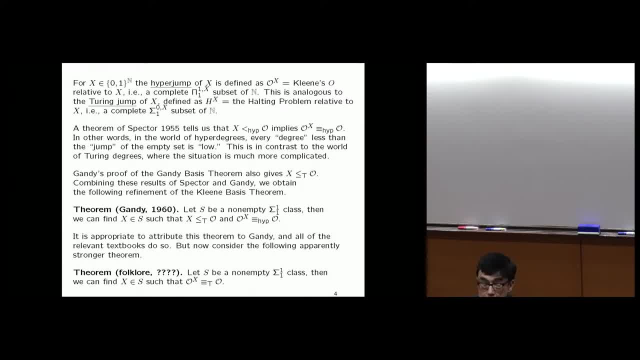 It's, it could be bigger than the halting problem, Right I mean. so here's zero and zero prime, the halting, the Turing degree of H. there are degrees in here, A, such that the jump A prime. 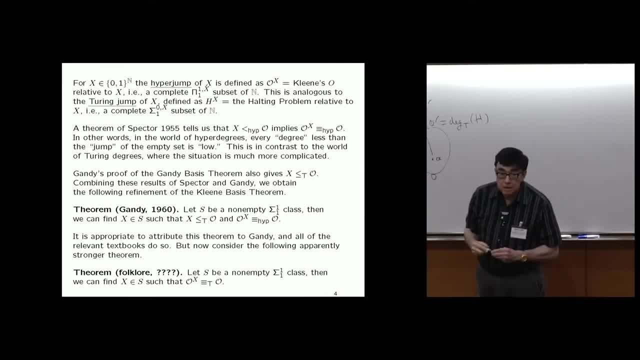 is, you know, out here, somewhere bigger than zero prime? There are things like that. but in the world of hyper-degrees, if you have any degree here and let's just call it the hyper-degree of the hyper-degree of, 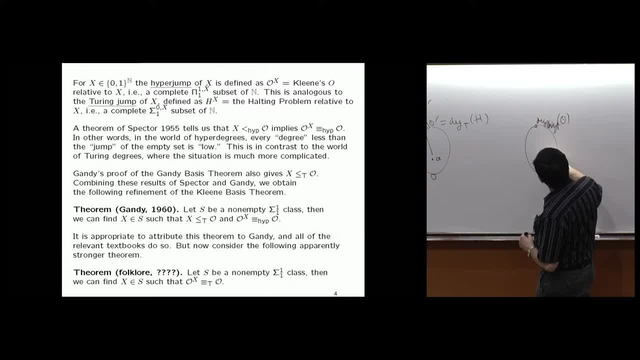 of O, the jump has to be. well, let's say, let's say this is the hyper-degree of X, then this has to equal A prime, in other words the hyper-degree of OX. There are no. every degree is low. 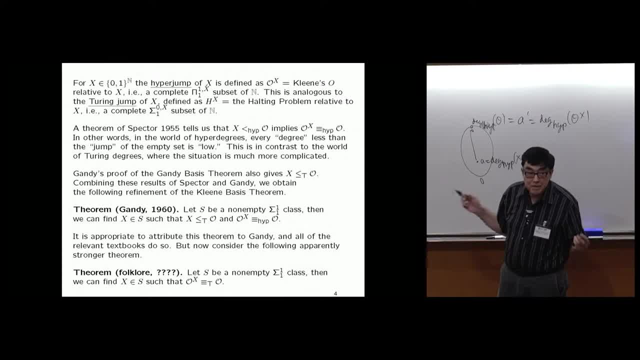 this is in the world of hyper-arithmetic theory. every degree is low. Every degree less than O. Kleene's O is low. So so that you know. in other words, the situation is much more complicated in the world of Turing degrees. 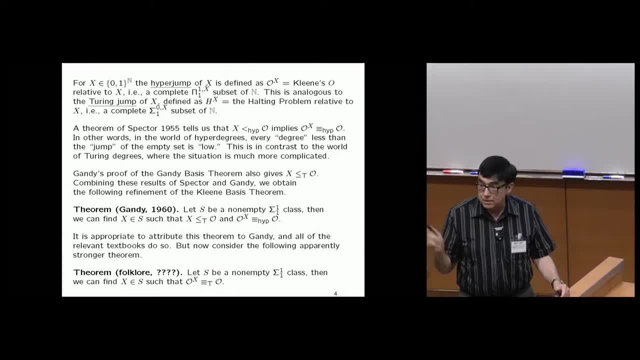 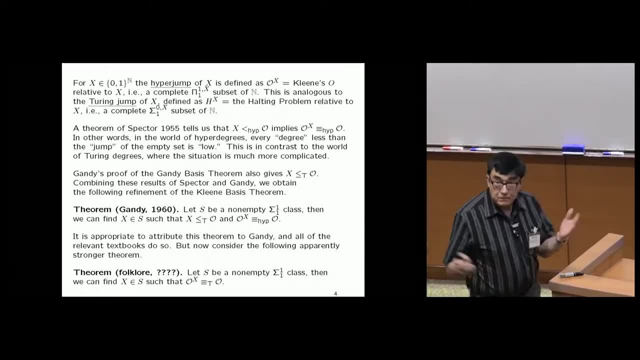 There are low degrees, high degrees, you know, low two, high two, et cetera, all kinds of things. So hyper-arithmetic theory. I've always thought that it's sort of simpler than recursion theory in some ways. 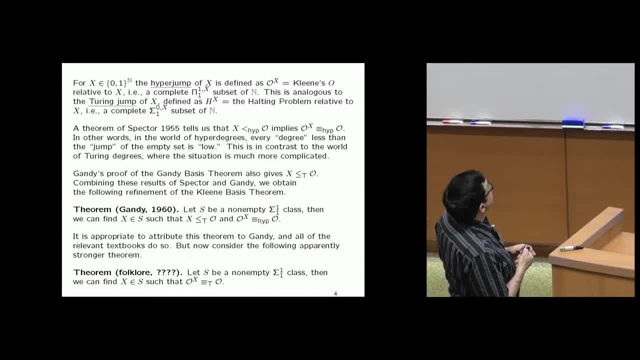 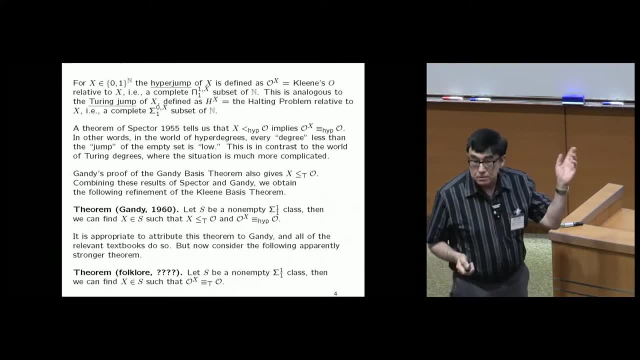 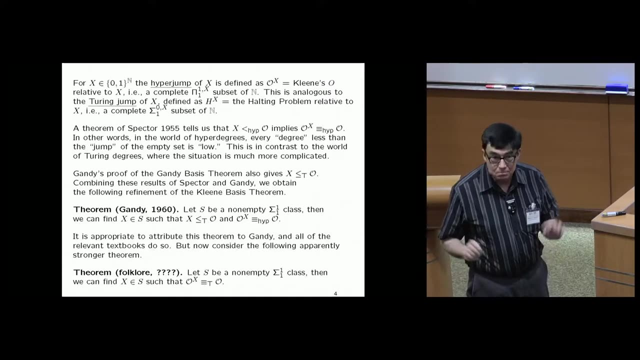 All right, yeah, here I'm trying to say that in this paragraph. By the way, these slides are available on my web page and so on. I'm going to revise them after, after I go home, but there is. what I'm showing you is. 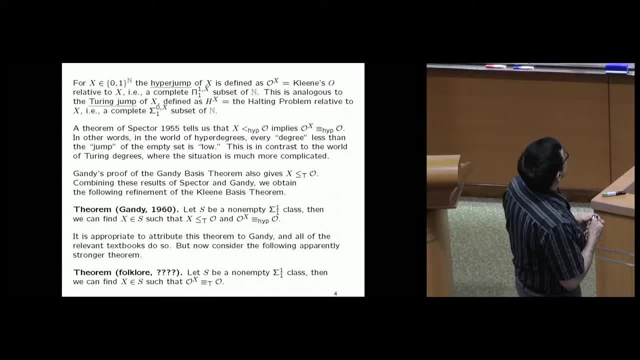 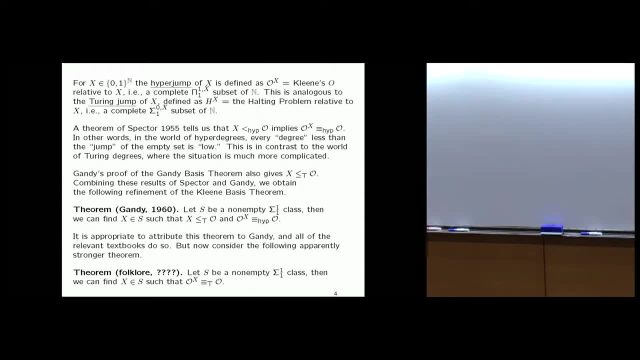 is there on my web page now. Okay, now Gandhi's. so that's a theorem of specter. So that has implications, because Gandhi basis theorem says there's a member of S which is of strictly lower hyper-degree than O. 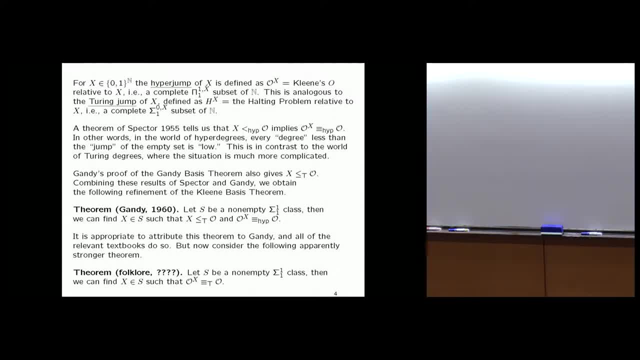 then it follows that X is hyper-arithmetically low. But another another piece of information implicit in Gandhi's proof of the Gandhi basis theorem is that X is Turing reducible to O, So Turing reducibility comes into this also. 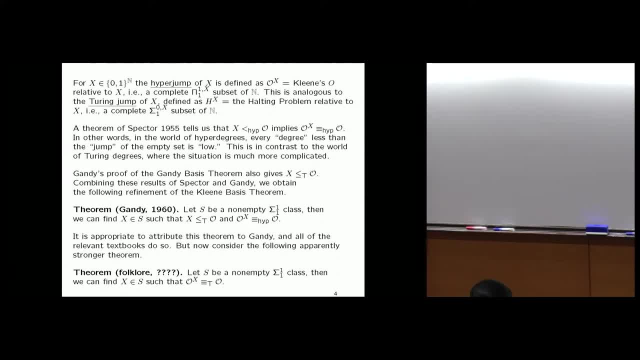 And because, in other words, he proves it by using the Kleene basis theorem and gets it recursive in O that way. So so, combining that you get this statement here, which I'm is property, would tribute to Gandhi. 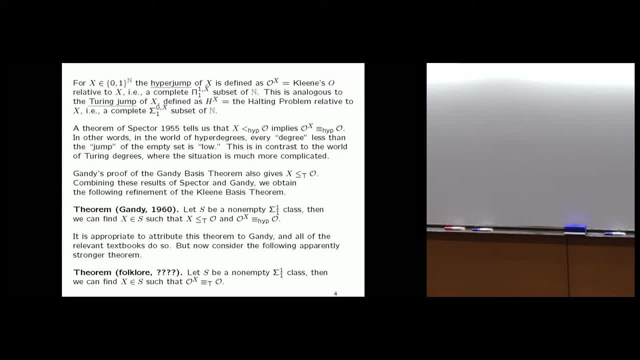 Let S be a non-empty sigma. 1, 1 class, then for some X in S X is Turing reducible to O and hyper-arithmetically low It's the hyper-jump of X is hyper-arithmetically equivalent to O. 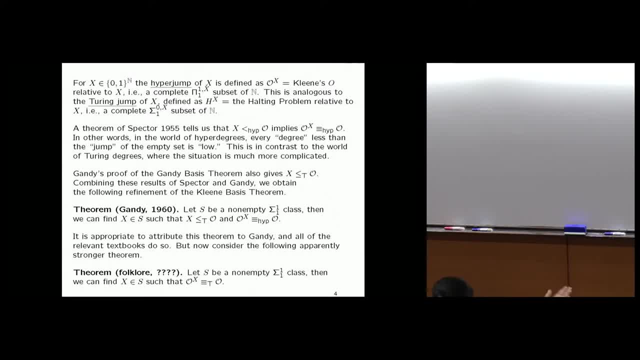 I I should say this is these, these Kleene basis theorem and Gandhi basis theorem. they're examples of basis theorems. A basis theorem is a theorem that tells you if a certain kind of nicely describable set is non-empty. 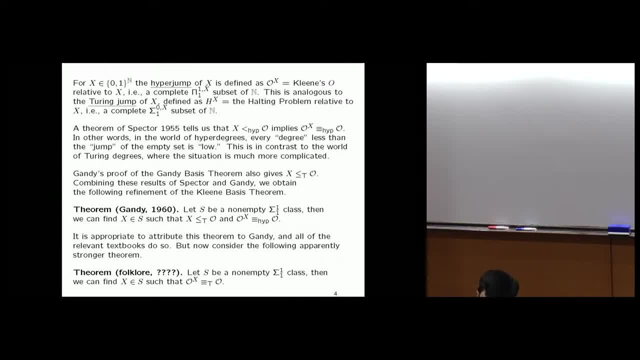 then it has an element which is also nicely describable in some way. Then there's these. these basis theorems are very important foundationally because a lot of foundations, a lot of foundational programs in mathematics had to do with you know. 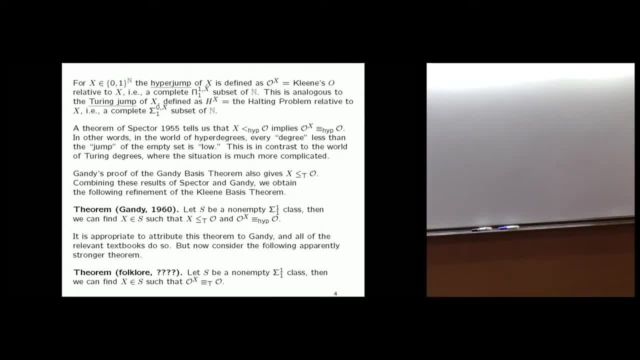 questioning whether we need to really have all these very complicated sets. Can we get away with just simpler sets, you know, and and so? so it's nice to know that if, if there is a set with a certain property, then there's a simple set with that property. 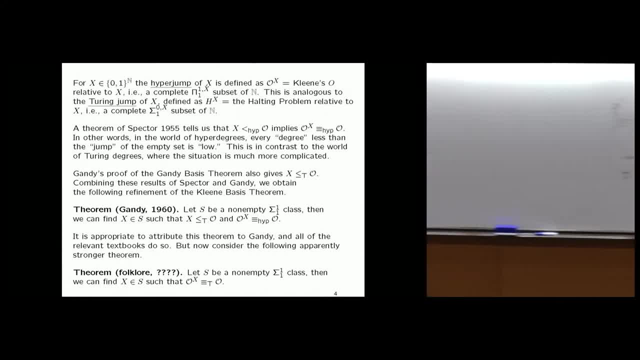 There's, you know, a nice, nice set, All right. So that's the Gandhi basis theorem, Really a combination of specters and Gandhi's result, And it's appropriate to attribute this to Gandhi and all of the relevant textbooks attributed to Gandhi. 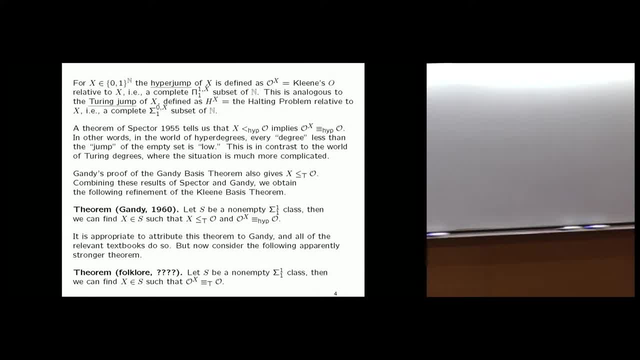 But now look at this other theorem. Let S be a non-empty sigma in one class, Then for some X in S, the hyperjump of X is Turing equivalent to O. So this is: this is hyperarithmetically low in a stronger sense. 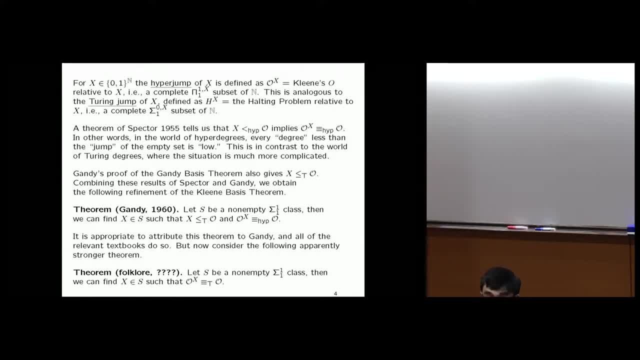 Not only is it hyperarithmetically equivalent to O, but it's Turing equivalent to O. Okay, That's, that's, that's a, a refinement, That's a, that's a. I say there that it's an apparently stronger theorem. 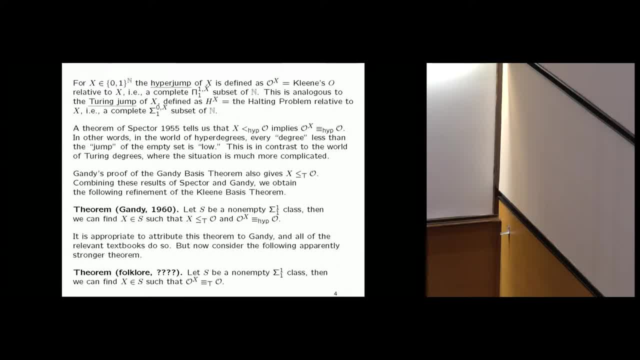 as I will remark on the next slide, or maybe one or two slides from now. It's actually. it actually is a stronger theorem. I'll explain. I'll explain So, but you know, on the face of it, I mean this property. 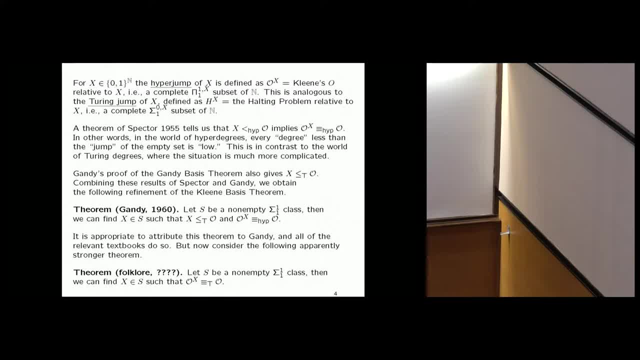 that the Turing, the, the hyperjump of X, is Turing equivalent to O implies both of these properties, that it's X itself is Turing reducible to O, and OX is hyperarithmetically equivalent to O. That's implied. 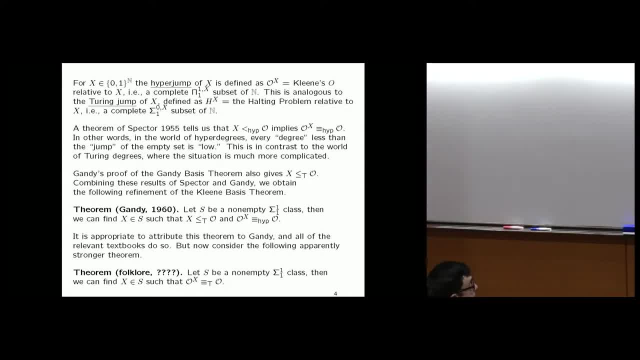 right. So so this is a but, but you don't. you know, there's a question of: is this equivalent to this? And the answer is no, it turns out as you would expect, All right, so. 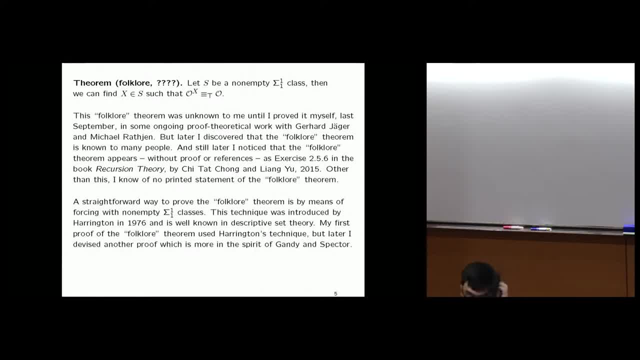 so there's this theorem. I'm just calling it a folklore theorem. What happened to me was last fall. I was doing some work with Gerhard Jaeger and Michael Rathjen. They're they're German proof theorists And they, they 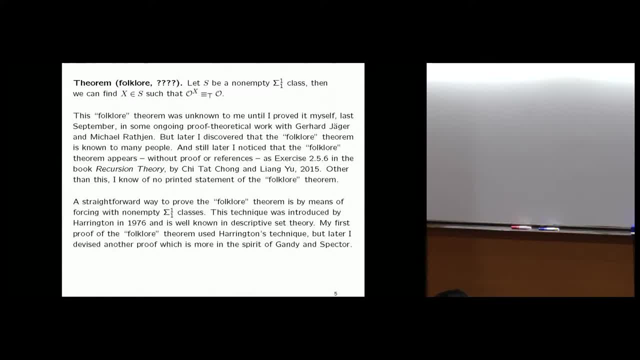 I. I came up with this folklore theorem Because it was relevant to what we were doing, And I proved it. I I thought, oh, I know how to, I can. I think I can prove that And I proved it. 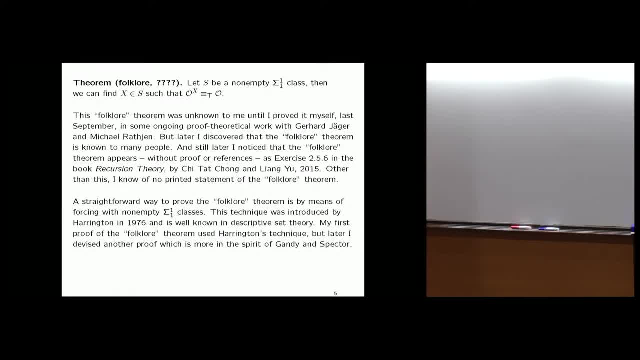 And and and then. but then I asked around later and I found out that this is known to many people, And so, to my surprise, I found out that many people just call this the Gandy basis theorem. They: 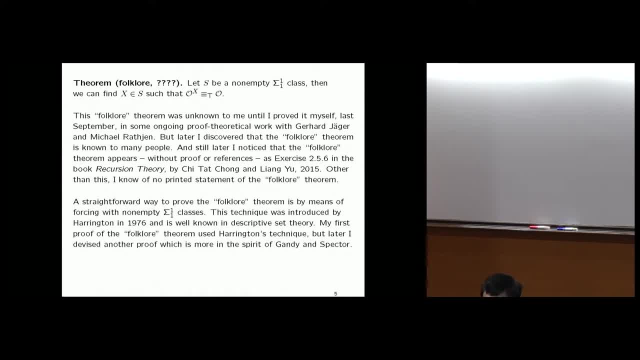 but it's. it's not there in Gandy's paper, And and so so I was trying to figure out what, what, what is the history of this theorem, What? that's why the question marks indicate I don't know where this came from. 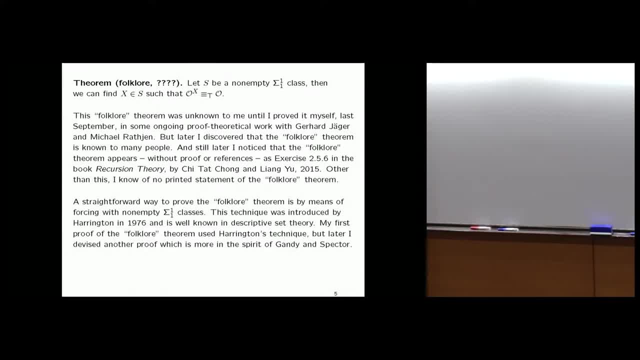 Who? who first proved this How it's? it's a folk. it seems to be folklore. A lot of people know it. I'm, I'm see. in fact, it sometimes seems to me I'm the only one who didn't know this. 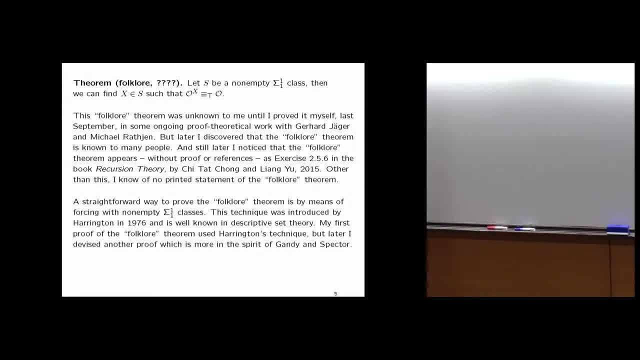 But. but. but there it is It. it appears, as I said, in in the, in the book by Chee Todd Chong and Liang Yu recursion theory, their recursion theory, their, it's really a book on hyper recursion theory. 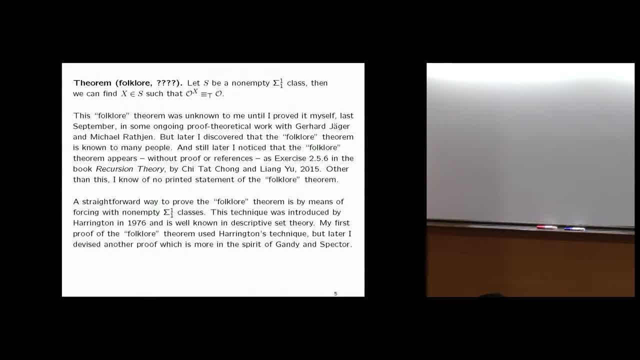 higher recursion theory. They actually stated as an exercise, but with no proof or references, So they they're not saying where it came from And okay, it's, it's, it's true, It's, it's, it's. 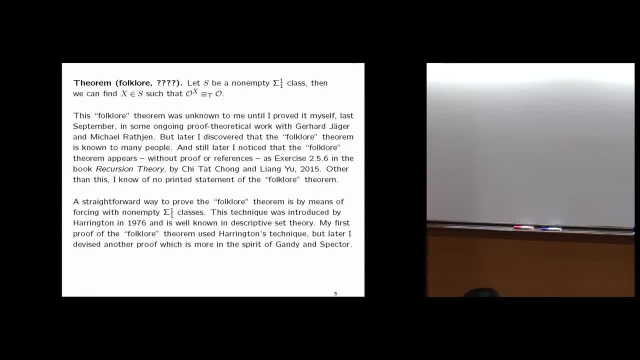 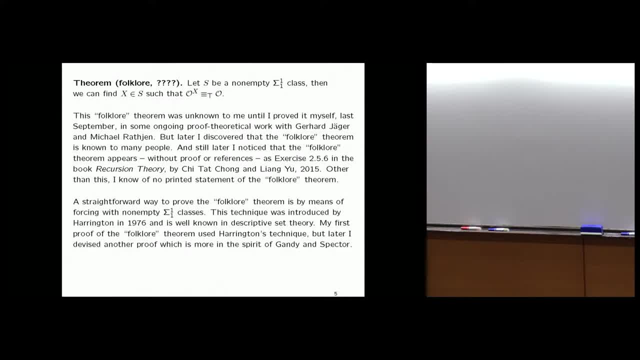 So now, how do you prove this thing? Well, you prove it by means of forcing. the easiest way to prove it to me is forcing with nonempty sigma one one classes. That's a technique that was introduced by Leo Harrington- by Leo Harrington in a manuscript in 1976.. This is one of Leo's unpublished manuscripts that are: 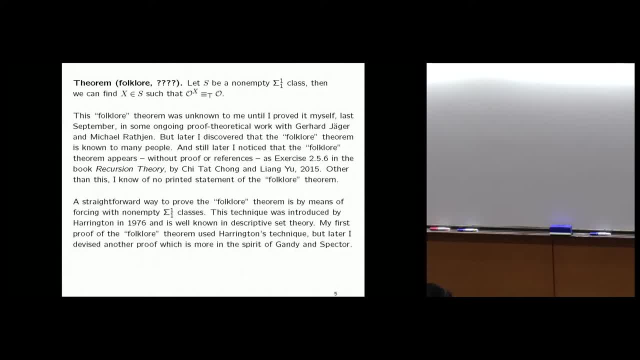 very basic to mathematical logic And this technique was introduced by him. It's well known in descriptive set theory. He used it to prove to give a. the title of the paper is a powerless proof of a theorem of silver. This is a theorem in descriptive set theory. 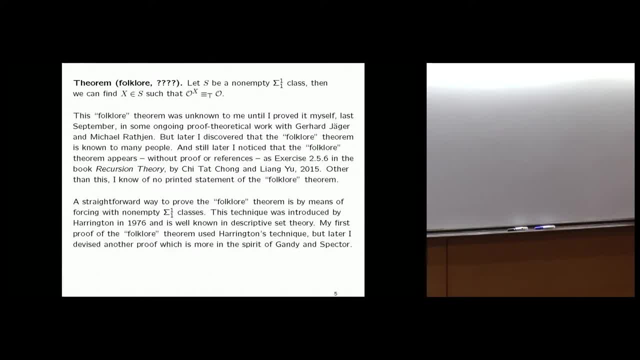 about analytic equivalence relations. So it's well, it's known in descriptive set theory. now I knew about it just because you know. I was in contact with Leo Harrington at the time And my first proof of this folklore theorem used Harrington's technique. Later I have another. 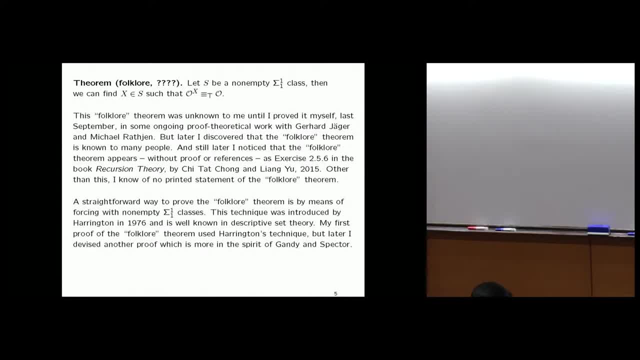 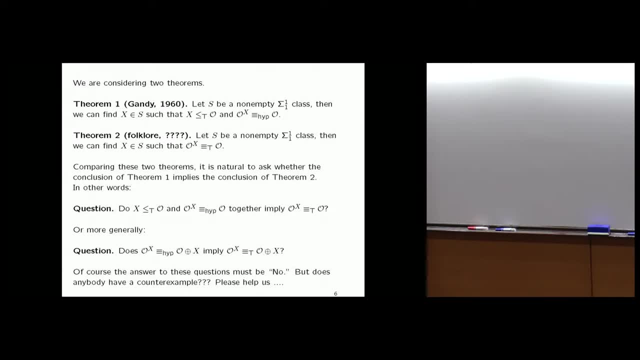 proof Which is more in the spirit of Gandhi and Specter. But it's not. it's just not there in Gandhi's paper. So so let's compare these two theorems. Here's Gandhi's theorem And here's the folklore. 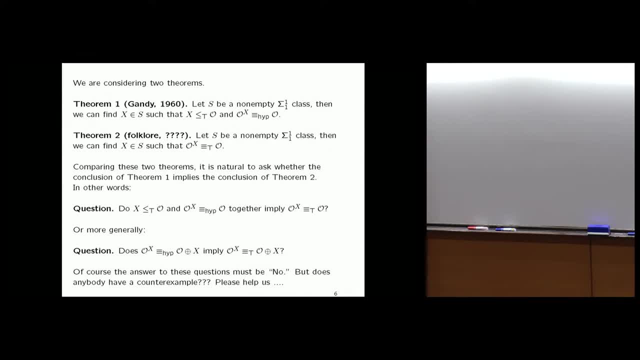 theorem, And it's natural to ask whether they're really the same theorem in the sense that the two conclusions are equivalent. Is it true? is? is the conjunction of these two properties, x Turing reducible to O and its hyperjump is hyper-rhythmically equivalent to O. is that? is that equivalent? 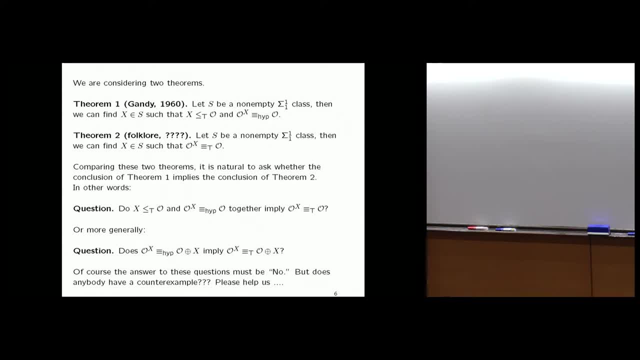 to just saying the stronger statement that the hyperjump of O, of x is Turing equivalent to O. So does do these, do these two conditions imply this other condition, You know, the difference being that here we have hyper-rhythmic equivalence? 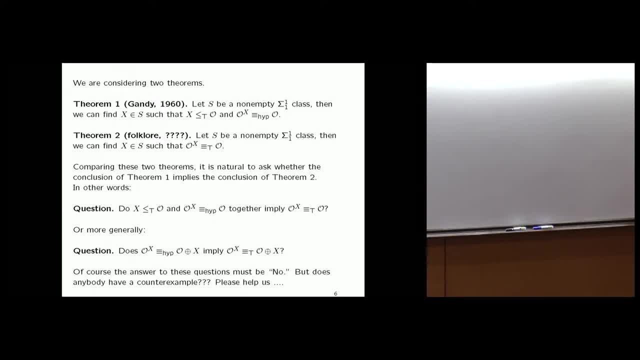 and here we have Turing equivalence. Or, more generally, if x, if we don't assume that x is Turing reducible to O, but we do assume that x is hyper-rhythmically low, generalized low, let's say generalized low in the sense of hyper-rhythmically low. 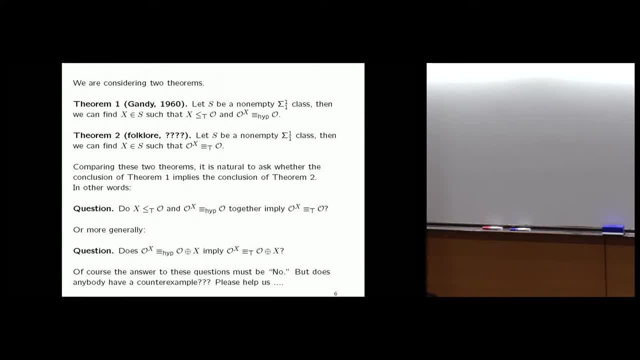 And then we have hyper-rhythmic theory: O- x is hyper-rhythmically equivalent to the joint of O and x. Is does that imply that it's Turing equivalent to the joint of O and x? Well, and you know, when I wrote these slides I thought the answer is no, but I didn't, I didn't know. an example. 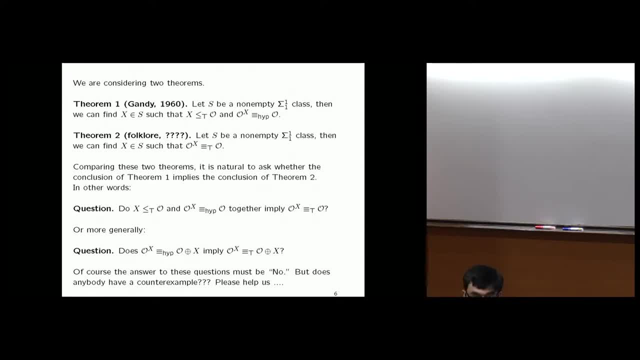 So I put these slides up and within a matter of a day, Ted Slayman emails me and says: oh sure, I have an example And he came up with an example. So great That's. that's this is. this workshop is really solving a lot of problems for me already. 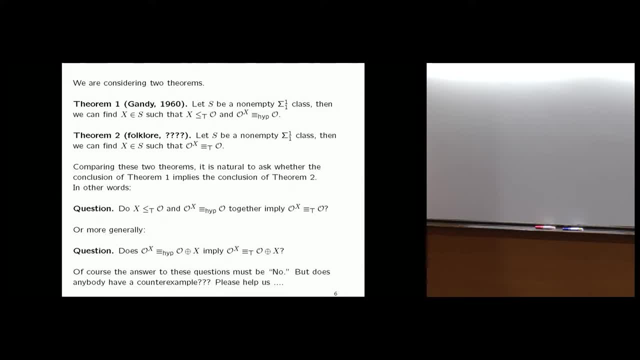 So please help us. Ted said, okay, I'll help him out, you know All right, So so so what Ted pointed out is that if you, if you do Sach's forcing, that is, you force with perfect closed sets in the, in the world of hyper-rhythmic theory. 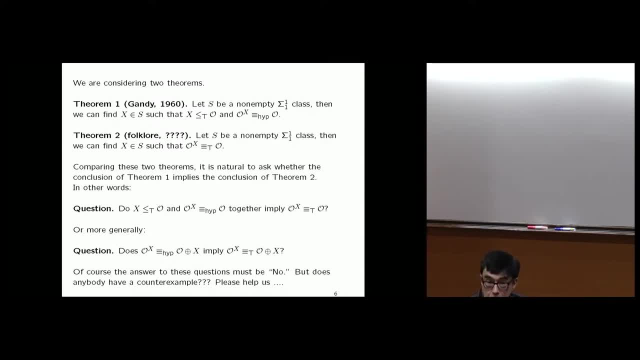 you get a real x. you know any sufficiently generic real in that sense of forcing will be- will be a counterexample to this. In other words, it'll it'll be hyper-rhythmically equivalent to O plus x, but not Turing equivalent to O plus x. 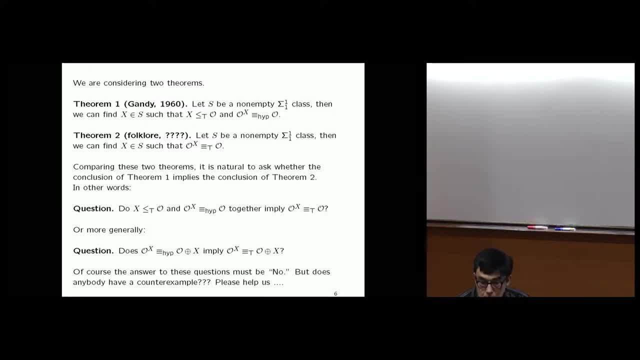 And you know, we, we can, I mean Ted can explain it to you, or I can explain it to you And, and, and Ted now tells me that. Ted also told me that it's also a counter you can also get using a similar method. 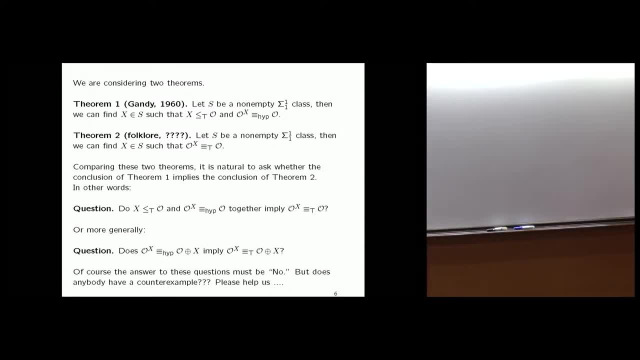 you can also get a counterexample to to the first question. That's a little harder. but he, he thinks, he, he, you know, I'm, I'm. I hope, I know, I hope I understand that before the end of this conference. 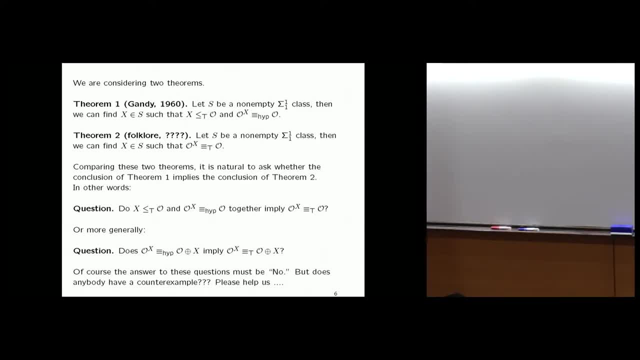 This workshop. Okay, so that's where we are with that. So this is not so. I just want to say this: this Fokler theorem is not the Gandy basis theorem- for those of you who call it that, It's not. it's just not that. 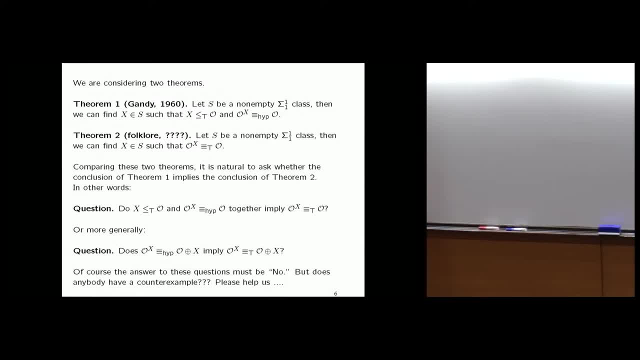 It's, it's. it's not quite what you, Leo, told me. I asked Leo about this and he said: well, yeah, maybe it's not the Gandy basis theorem, but we should have a lot of respect for Gandy. 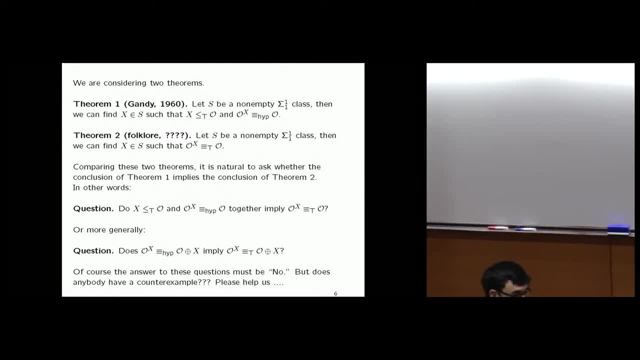 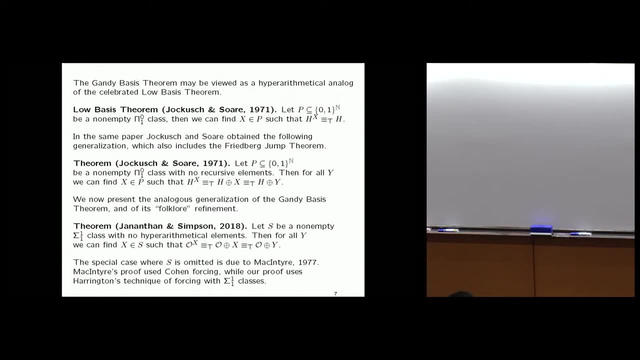 I do, I have a lot of respect for Gandy, It's just, You know. So, okay, Just the history. So the the, the Gandy basis theorem may be viewed as a hyper. now, okay, now I want to make another comment. 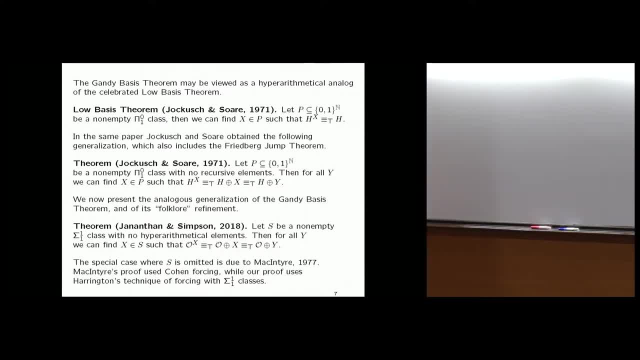 about something related to the Gandy basis theorem. The Gandy basis theorem is analogous to a well-known theorem in recursion theory. It's it's a hyper-arithmetical analog of a well-known recursion theory theorem- basis theorem, which is called the low basis theorem. 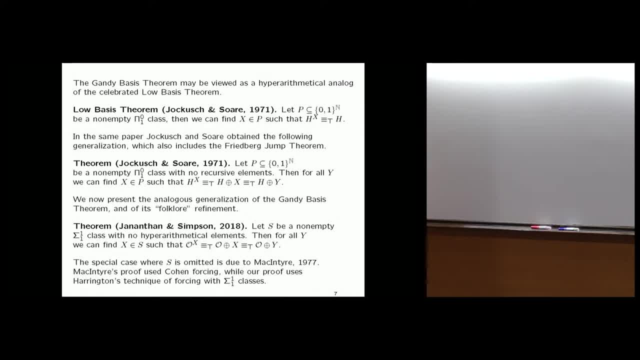 So let P be a non-empty pi zero one class. Then we can find X in P such that the Turing jump of X- H, the halting problem relative to X, is Turing equivalent to the halting problem. That is exactly the same statement as the Fokler theorem. if you replace pi zero one by sigma one one. 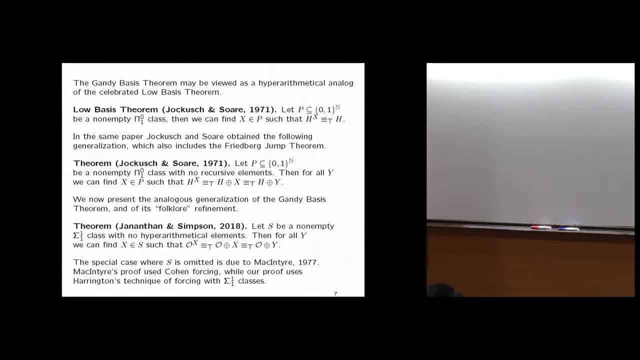 and you replace H by O, the hyper jump Instead of Turing jump and the halting problem. you'd have the hyper jump and Kleene's O. It's exactly analogous to that And what you're still using in the Fokler theorem: you're still using Turing equivalents. 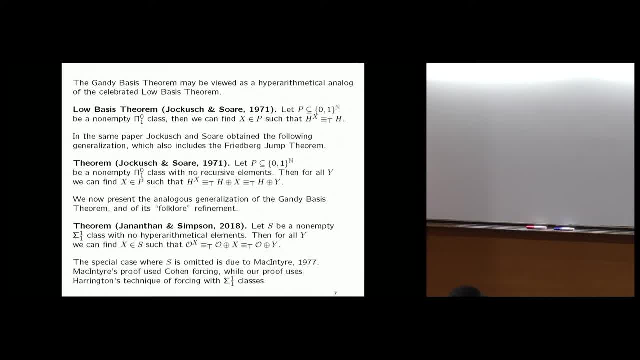 Now, Yes, yes, it did, but just intellectually it's analogous. Well, analog doesn't mean necessarily it came first. Usually people talk that way, but, like you know, it's a copy of it. It's not a copy of it, because all right. 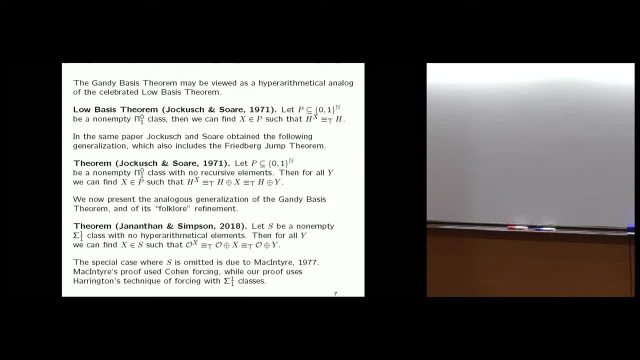 Anyway, In that same paper Jakesh and Soar also proved this generalization of the low basis theorem. It's not well known, but it's not what. 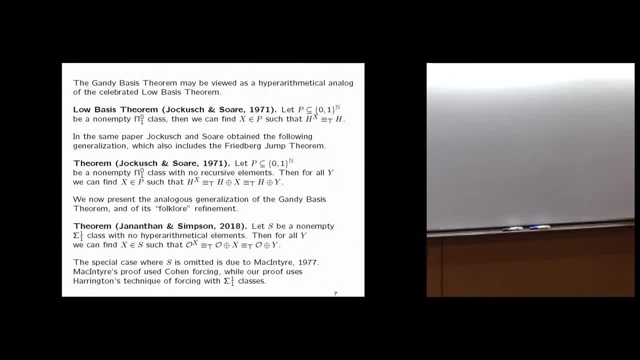 non-empty pisor, one class with no recursive elements. you can find members of that class which have whose jump is any Turing degree. 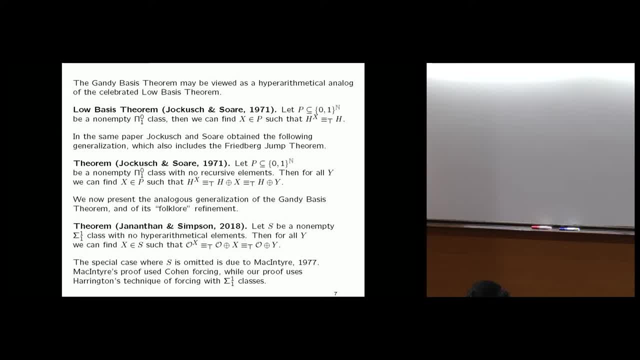 that you want, basically Any reasonable Turing degree, Any Turing degree above the halting problem. So that's there in their paper. And now I want to present the analogous. now this is an analog because it came much later- The generalization of the Gandy basis theorem. 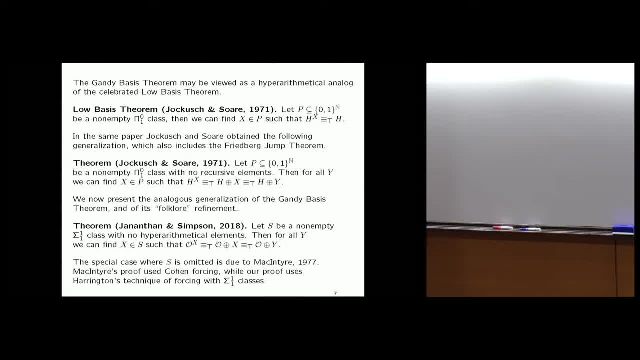 and its folklore refinement. so this is something that Jenanthan and I approved. Let S be a non-empty sigma, one, one class with no hyper-arithmetical elements. then for all Y, we can find an X in S, such that the same thing happens. 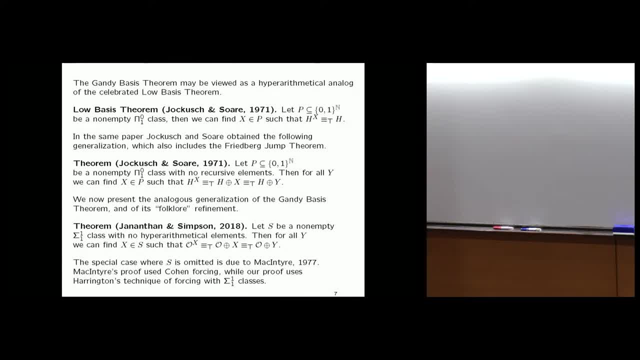 with Turing jump replaced by hyper jump, A halting problem replaced by O And uh. so that's it, It's just. it's just exactly analogous to their theorem, But with Turing reducibility, not hyper-arithmetical reducibility. 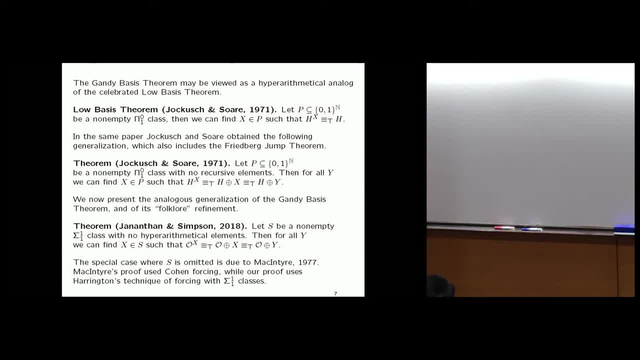 By the way, Turing reducibility is the master, is the most important kind of reducibility in my opinion. And you know, the hyper jump is just the omega one, CK jump, That's what it is, In other words, 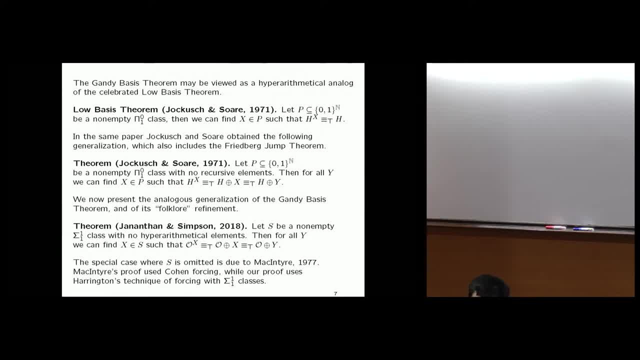 it's, the hyper jump of X is the omega one to the X jump of X, And it's, it's a Turing degree. really. It's well defined, the hyper jump is certainly well defined up to Turing degree, And, and I mean if two things are hyper-arithmetically equivalent, 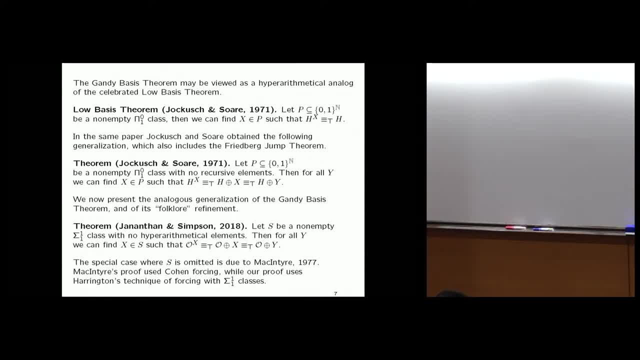 then they have the same. their hyper jumps have are the same, up to Turing degree. So, um. so we proved that. uh, the proof is not difficult, It just uses Harrington's technique again. Uh, the special case where S is omitted. 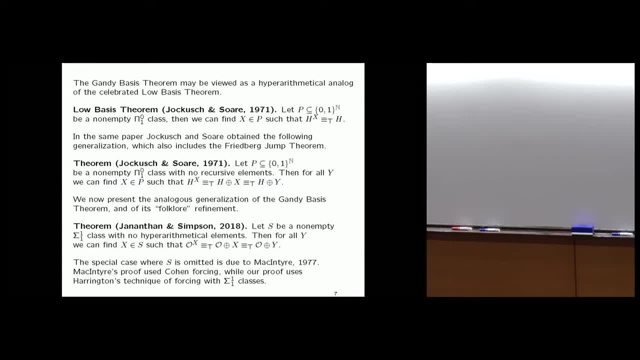 if you just say for all Y there exists an X, such that, uh, this conclusion holds, and just ignore S. that was proved earlier by another uh uh practitioner of higher recursion theory called John McIntyre- I understand Angus McIntyre is gonna be at this. 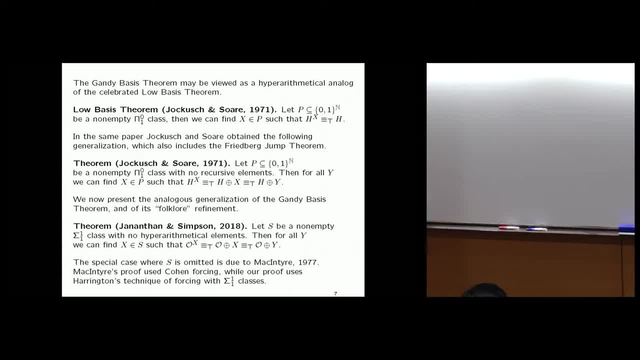 uh, here, be around here this summer. right, He's, yeah, but uh, uh, this is. this is not Angus McIntyre, It's John McIntyre. Um, and and uh, he, his proof used Cohen forcing. 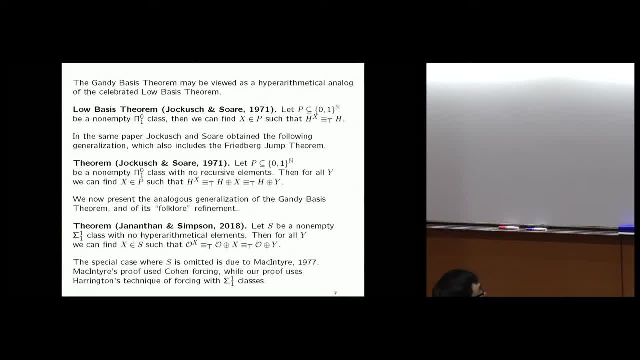 It's published in the JSL Um, and our proof, of course, uses Harrington's technique of forcing with sigmoid force, So so uh, uh of the of the hyper-rhythmetic, uh analog, So uh. 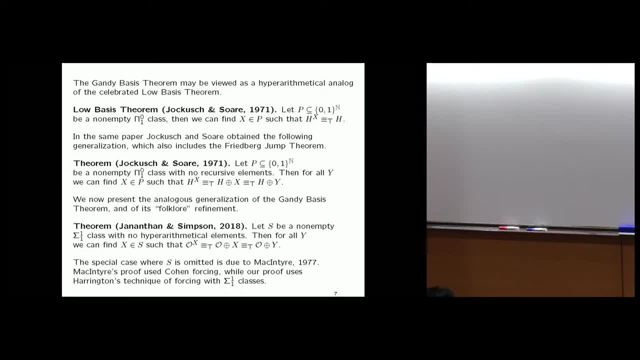 so there's, uh, there's. that, That's one thing we did, All right, uh, so, uh, all right. so so much for the Gandy basis theorem and related theorems I I've already taken up uh. 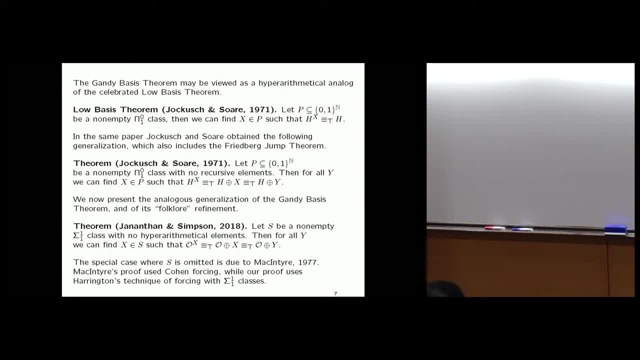 half of my time I think: All right, now let's go on. So uh, so, this made us think. you know what, what other basic theorems see? in other words, let me uh, just this: the the Turing degree version of this is: 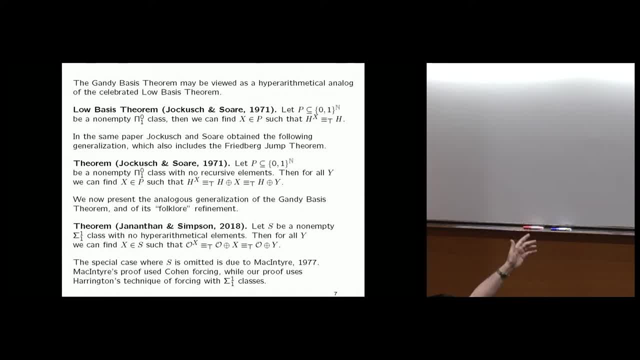 uh of this uh jump inversion is is just uh, Friedberg's jump inversion theorem. But there the jump, the jump operator, the Turing jump operator, has other well-known basic properties: The Posner-Robinson theorem. 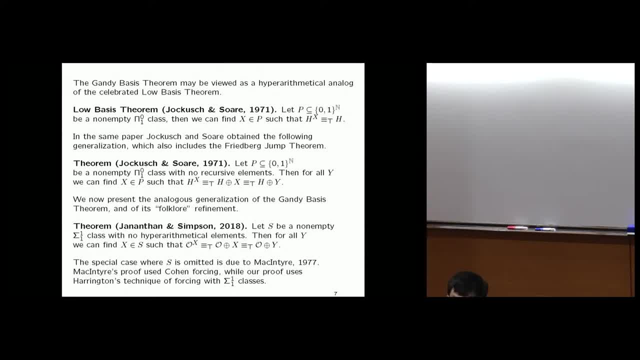 and there's something called the pseudo-jump inversion theorem. So, uh, these are very basic properties of the Turing jump, And, uh, I think of them that way. And what, uh, what, what? can we generalize those to hyper-arithmetic theory in a similar way? 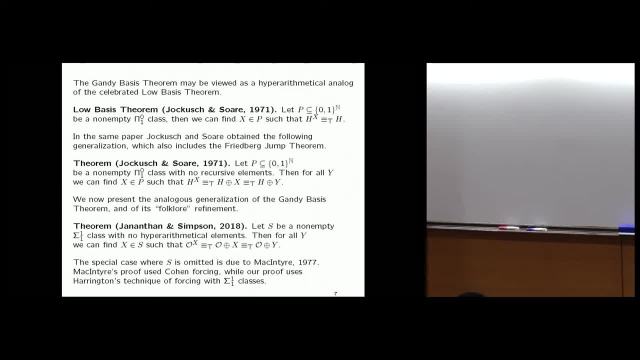 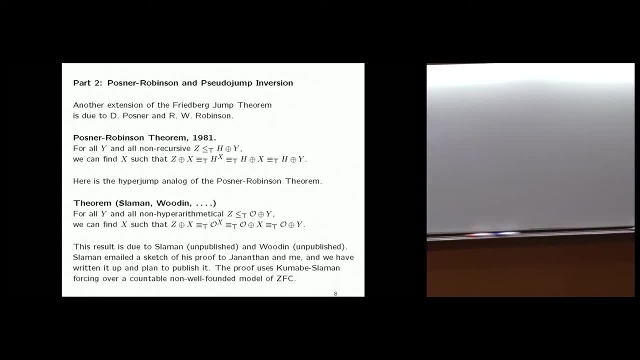 So, so, let's, let's look at that, And here we're mostly floundering, but, uh, we have some results. Uh, so another extension of the Friedberg jump theorem is, uh, the Friedberg jump theorem. 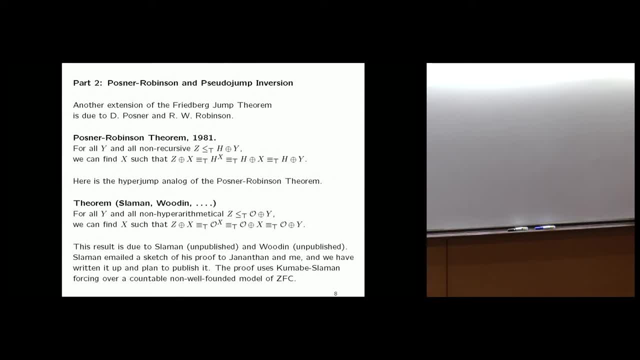 I should have stated it by now, the Friedberg jump theorem. but anyway, you know what it is. It's well, I'll- uh, I think it's stated on a later slide. Um, this is a theorem in 1981.. 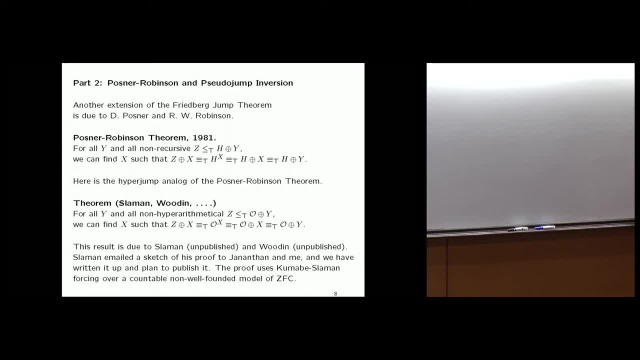 Basic property of the Turing jump operator for let let's. let's try to read this in an easy way. Start with let let Z be a non-recursive real, any non-recursive real, Then you can find an X. 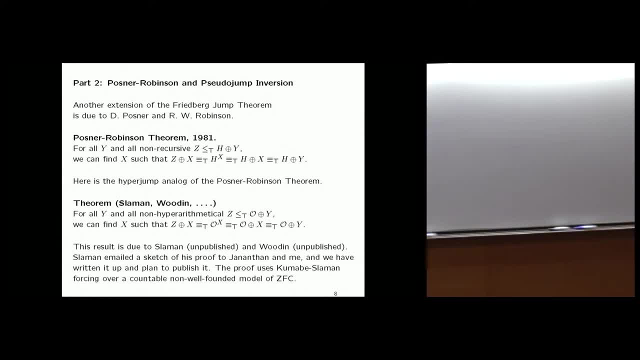 such that Z join X, that X joins Z up to the Turing jump of X, And you can make the jump, the Turing jump of X, be any Turing degree you want. Okay, That's, that's the Posner-Robinson theorem. 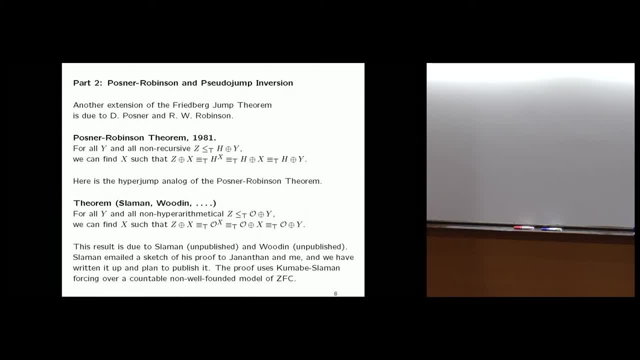 Um, okay, uh, now, and I state it this way just to make sure it's all stated correctly, but this is what it says Now. uh, we tried to prove the- uh- hyper-arithmetical analog. Well, first we tried to find out whether it's true. 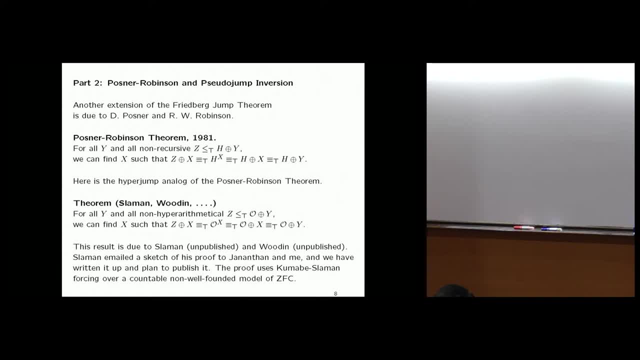 Um, it's sort of attributed to Wooden in different places, but Wooden, he proved a paper proving a, he he published a paper proving a related result, but not exactly this. And uh, uh about TT equivalence, Uh, 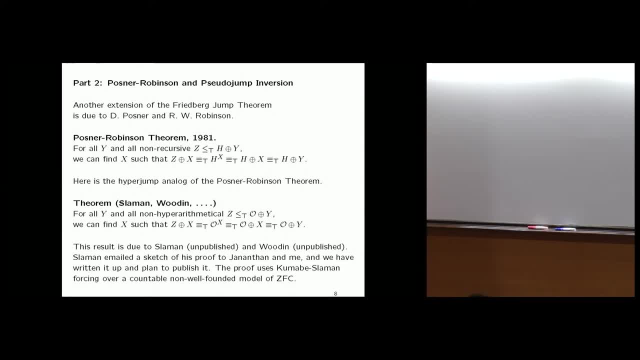 I I sorry I left that one out of the references here, but but that's you know, and and I guess he must be using the same method as in that paper to to prove this. But anyway, this is the hyper-arithmetical analog. 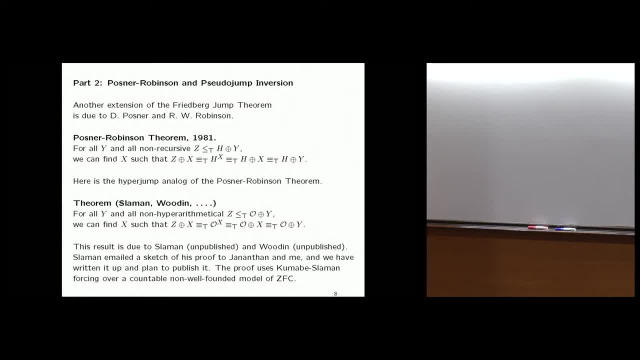 of the Posner-Robinson theorem For all. it. just replace non-recursive by non-hyper-arithmetical, and then uh replace the Turing jump or Kleene, uh, the halting problem by Kleene's O. 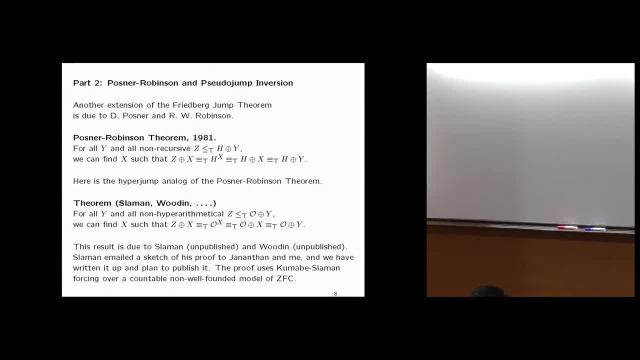 And that's it. It's the. it's completely analogous. Um so, uh, now this theorem we didn't succeed in proving. We tried to use sigma-1-1 forcing, you know the Harrington forcing, but it doesn't work. 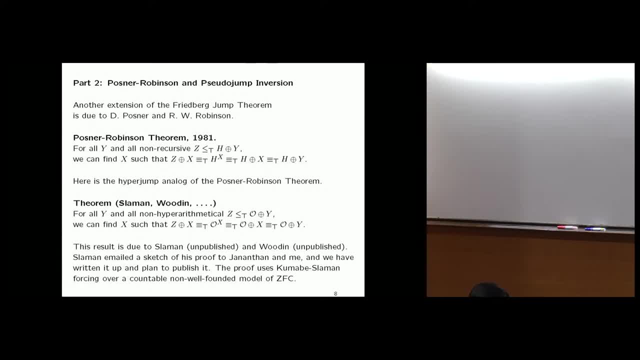 And um, uh, but. but we found these references and I asked Liang Yu and CT Chang about it and other people. uh, and they, they, they. they told me basically that Sleiman and Wooden knew. 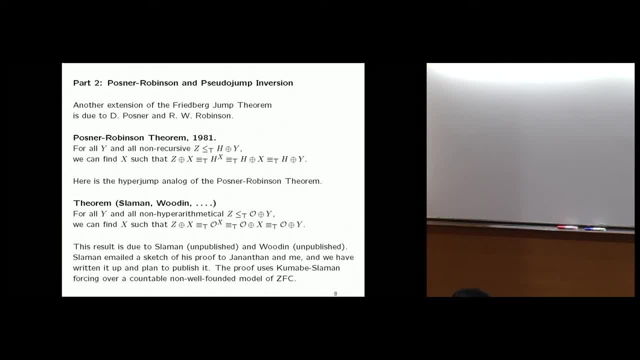 how to prove this. So I wrote to Sleiman and Sleiman said: said uh sent us his uh proof, a sketch of his proof uh, and we have written it up and we plan to publish it. 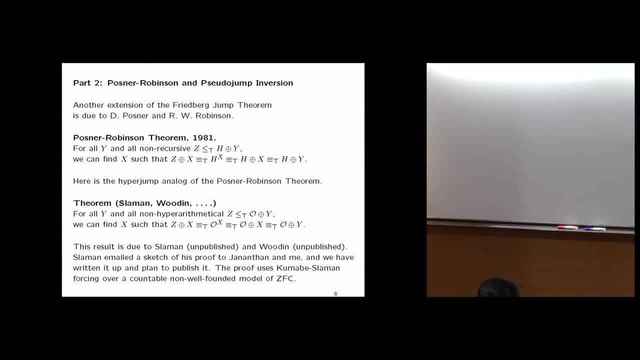 Uh, the the proof uses the same idea that he's used previously in generalizations of the theory, namely Kumabe-Sleiman forcing. Oh, Kumabe is also here in the, in the audience It's. this is a higher recursion. 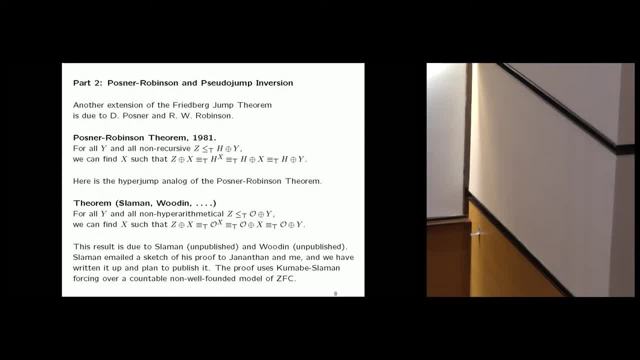 theory, uh, reunion here. Um, um, um, so, uh, so the and the interesting. an interesting aspect of this proof, as opposed to previous ones, is that it uses forcing. due to Sleiman's proof. 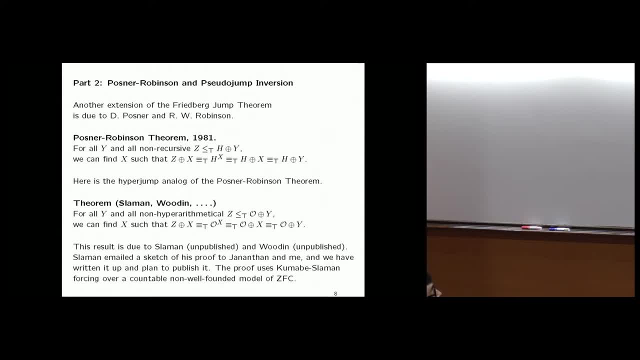 this is it's. it uses forcing. you know usually when, when you use forcing, you're forcing over a well-founded model of ZFC. you know accountable- usually accountable well-founded model. Here we're for forcing over a. 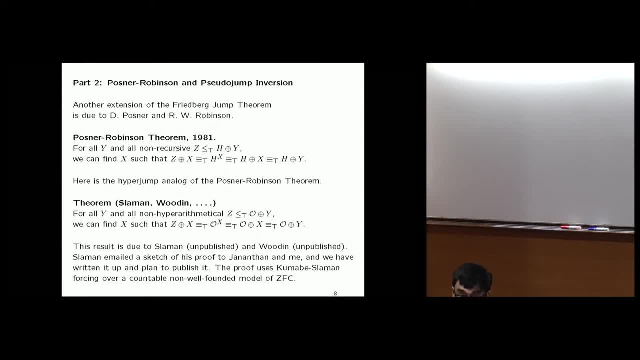 a accountable model of ZFC which is not well-founded. It's an omega model, but it's not well-founded. You have to do that to prove this theorem, So you need to check that all that forcing works over non-well-founded models. 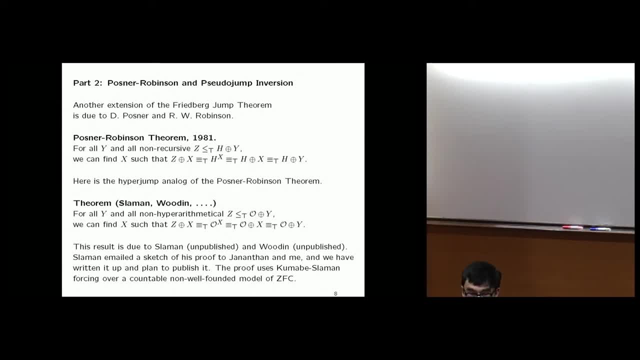 It just works. but you know it's, it's just not presented that way in textbooks. So so, so poor Jananthan had to, you know, go through all this. So so, so that's, but it's. 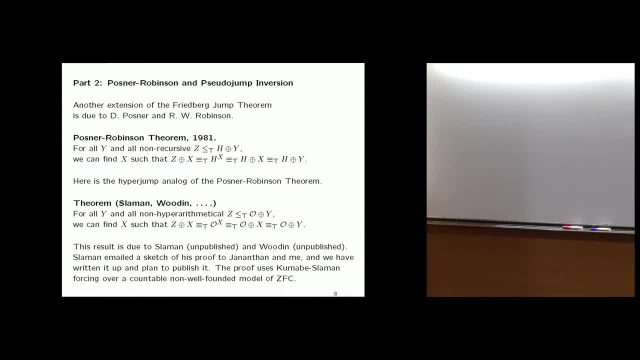 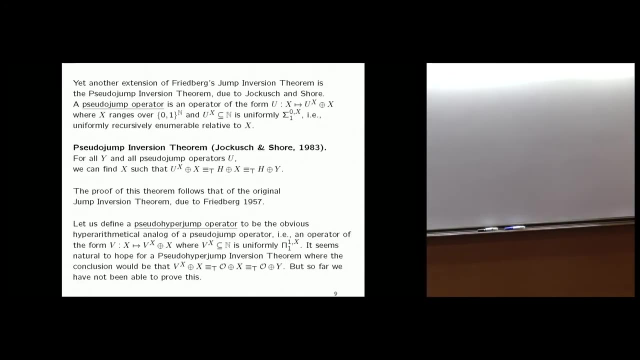 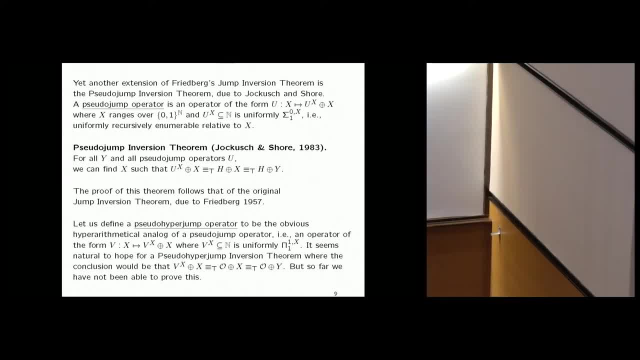 so, so, so, so, so. so what do I mean by a pseudo-jump? A pseudo-jump is also called an R-E-A operator, also called an R-E-A operator, also called an R-E-A operator if. 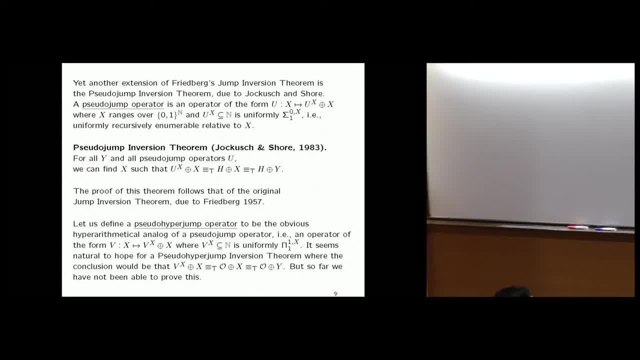 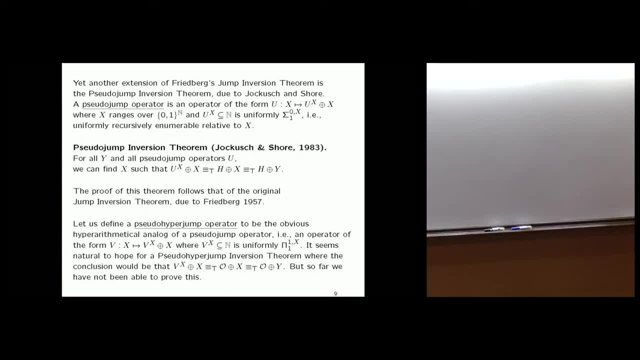 All right, it's so. ux is uniformly sigma zero, one and x and you have to throw x in. I mean ux might. if it's just sigma zero one and x, it may not actually include x as part of itself. 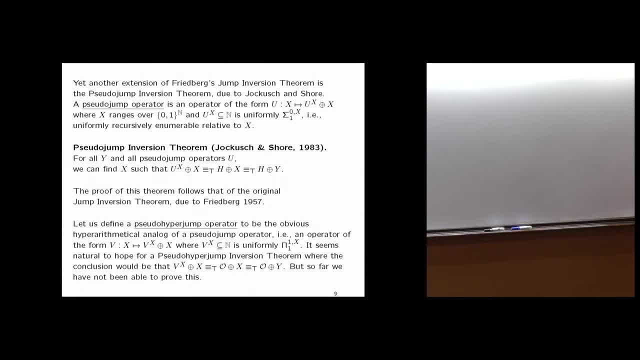 but we join it with x to make sure it does. So that's called a pseudo-jump operator and of course the standard example of a pseudo-jump operator is the Turing jump operator. Right, All, right now. pseudo-jump inversion theorem. 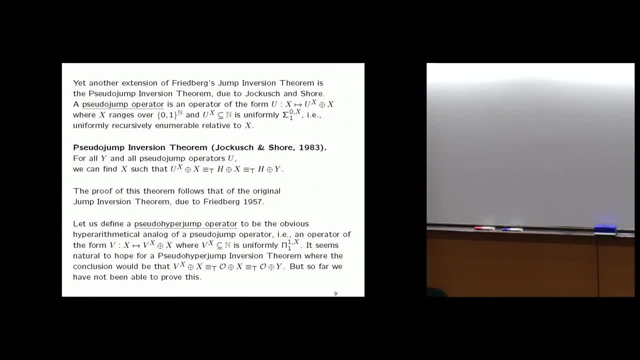 due to Jokic and Shor. not Jokic and Shor. is this: that for all y and all pseudo-jump operators u, we can find an x like this: that the pseudo-jump of x is equivalent to x. 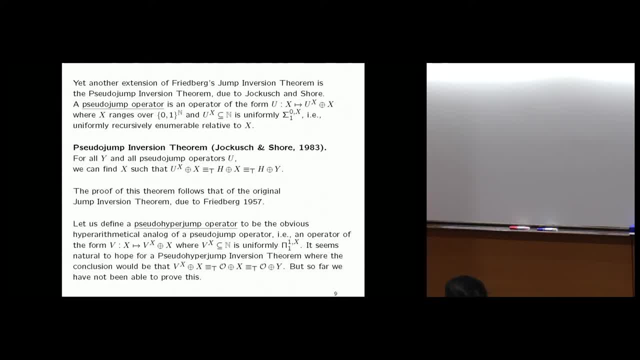 and it's anything you want it to be, above the, the Turing degree, above the halting Turing degree of the halting problem. So, and it's proved, exactly like the Friedberg jump theorem, You just imitate the proof of the Friedberg jump theorem. 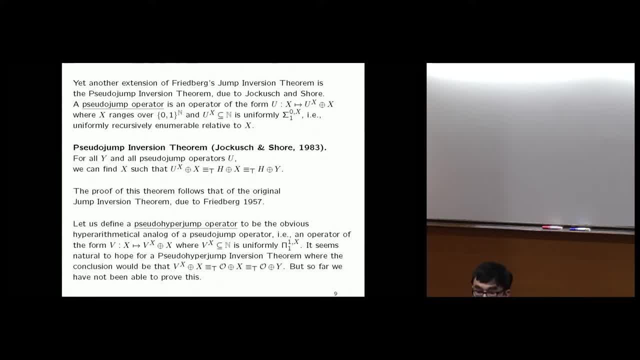 and it gives you this, But this is a powerful theorem. This is an interesting theorem and it has applications that the Friedberg jump theorem just doesn't have. So, and then there are variants and improvements of this and so on, But the proof of this is very easy. 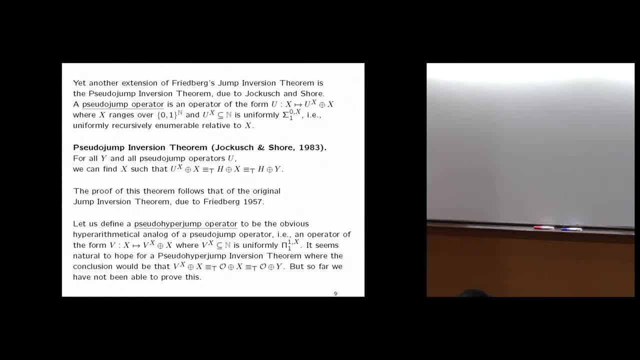 It's just the proof, basically the proof of the Friedberg jump theorem in just using a pseudo-jump operator instead of the standard jump operator. So so, as I say, it follows the proof, the original proof of the Friedberg jump theorem. 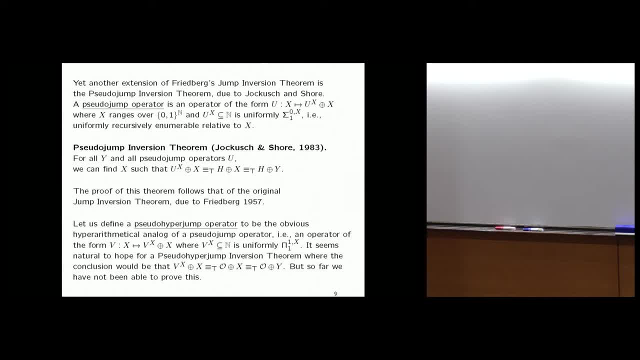 due to Friedberg 1957.. Now, so we want to know: okay, can you lift this? Can you? can you? is there an analogous theorem in hyper-arithmetic theory? So we define a pseudo-hyper-jump operator, to be the obvious thing. 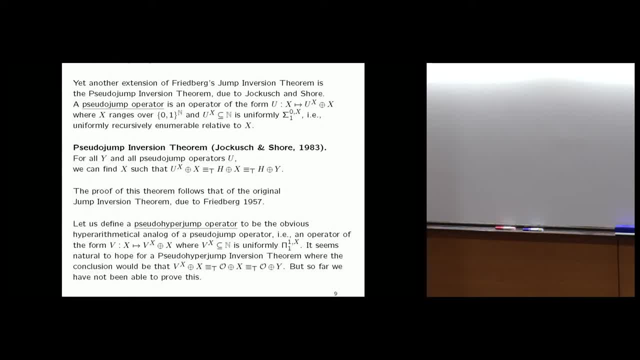 It's an operator which carries x to something, that's pi one one relative to x, and then join it with x to make sure it includes x, Pi one one being the analog of recursively enumerable. Okay, so it seems natural. It seemed natural to us. 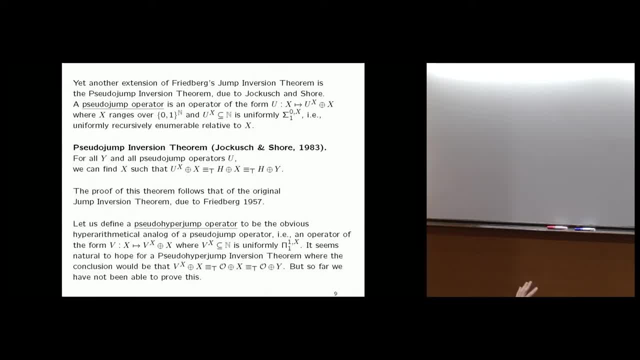 and it does. it still seems natural to hope for a pseudo-hyper-jump inversion theorem which would be just like this, except the conclusion would be vx plus x and would be, in other words, with this pseudo-hyper-jump operation, 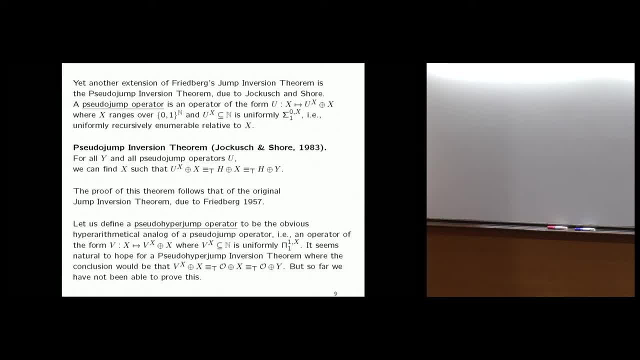 instead of a pseudo-jump operation, and Kleene's O instead of x. So that would be kind of the halting problem. It would be analogous, but we have not been able to prove that. That's where we are, Okay. 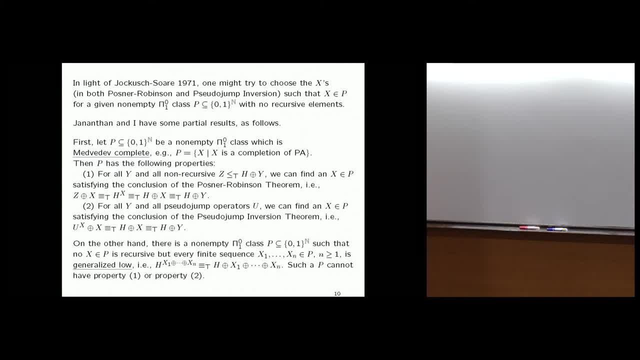 Now another question is that we thought about: was can you in these, in this, in the pseudo, in the Posner-Robinson hyper-arithmetic, the posner-Robinson theorem, can you choose x to be a member of a sigma one, one class? 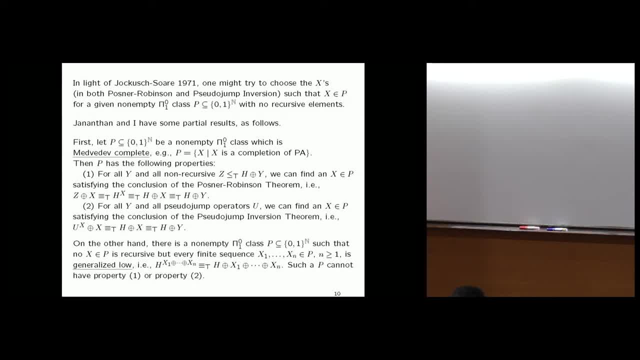 that you specify in advance. Well, and similarly for pseudo-jump inversion. except we don't know how to prove the hyper-arithmetic analog of. we don't know that that's true. We don't even know that this hyper-arithmetic analog 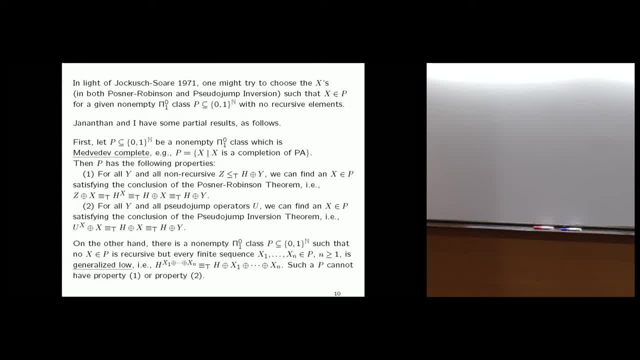 of pseudo-jump inversion is true, But if it is, can you ever? can you prove? can you get? can you improve the hyper-arithmetic? Okay, so we can, we can do that. Can you get? can you improve it? 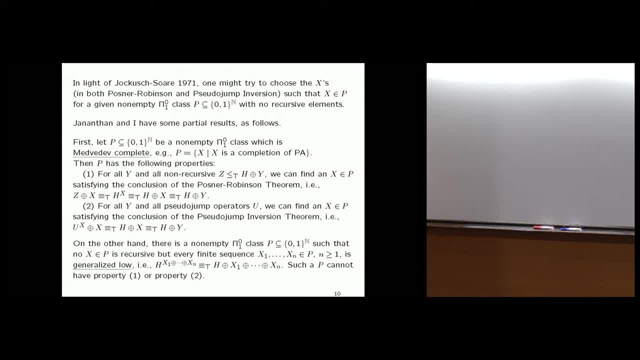 can you refine it further by getting by getting it to be a basis theorem. you know where you choose it from an arbitrary sigma, one, one class, And we have some partial results. in the Turing case This has to do with pi zero, one classes. 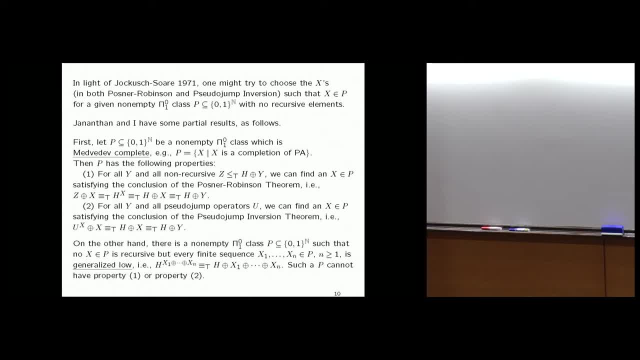 you know subclasses of the Cantor space. If p is a nice pi zero one class which is Medvedev complete, an example of a Medvedev complete class is the class of completions of piano arithmetic And actually all Medvedev complete, pi zero one classes. 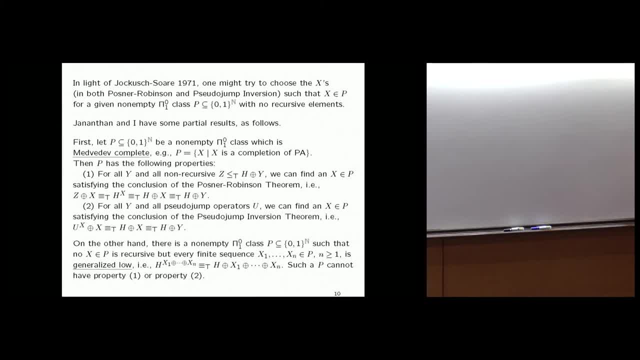 are recursively homeomorphic to that. So that's the only one essentially up to recursive homeomorphism. Then you can. you can choose your x in the Posner-Robbins the theorem to belong to that class And also in the pseudo jump inversion theorem. 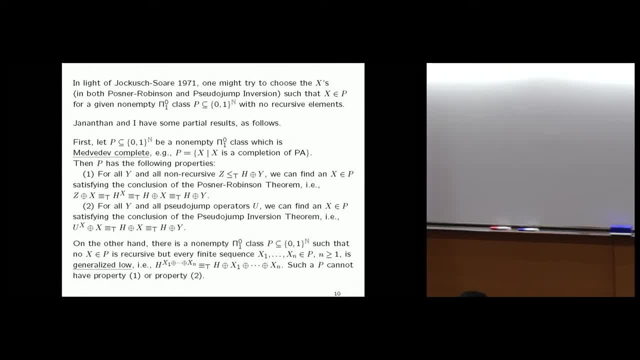 you can choose x from from that class. So that's that's. we do have those kinds of refinements. if p is Medvedev, complete. However, if if p is not Medvedev complete, we have a counterexample. 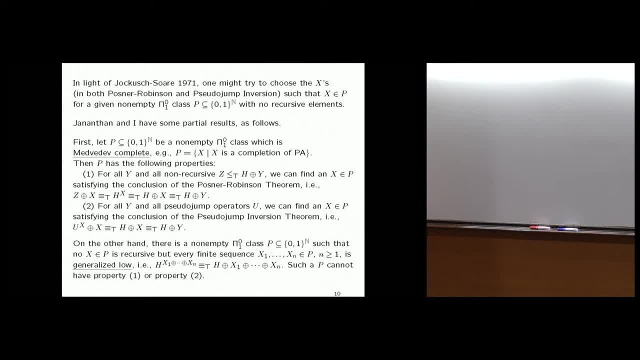 There is a pi zero, one class, such that that it's not empty. It no element is recursive. No, no, non, no recursive elements. But every finite sequence of elements of p is generalized low. Okay, that the Turing jump of the sequence. 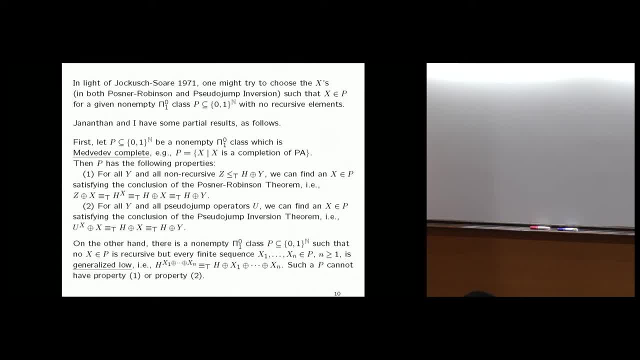 is equivalent to the join of the halting problem plus the sequence, And that's easy, That's not a difficult construction of a pi zero, one class, And such a, such a p cannot have, cannot. you can't choose x and p in this Posner-Robinson. 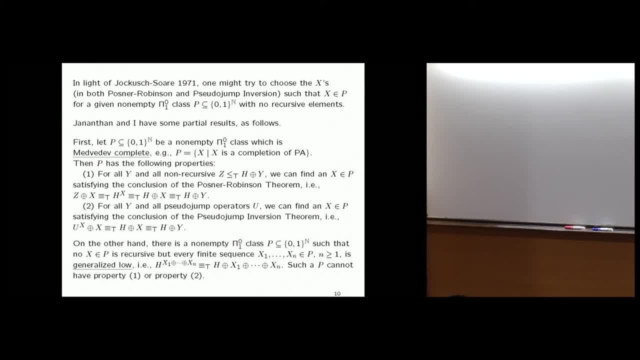 or in the pseudo jump inversion, Because you know you take one element of p, well the the other, any other element of p, is not going to be able to join to the halting problem, for example, It's not going to, its pseudo jump won't be the halting. 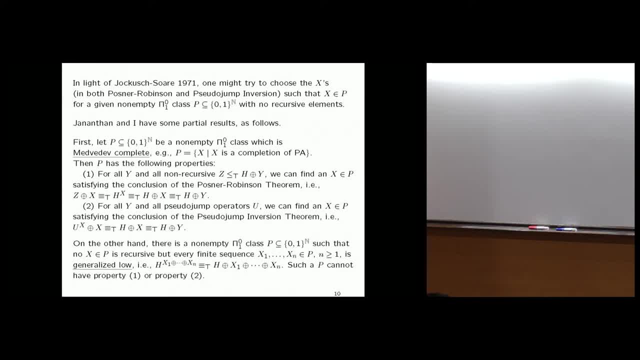 you know, it's just not going to work. So so that's a counterexample, But we don't know anything else, We, we don't, you know. and so an open problem would be to characterize the pi zero one classes. 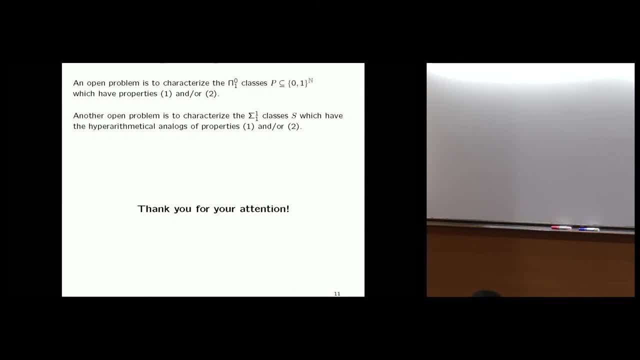 which have properties, one or two, That is, that you can choose the x for the Posner-Robinson or for pseudo jump inversion from p. And another open problem- even more open is because we don't have any examples- is to characterize the sigma one: one classes. 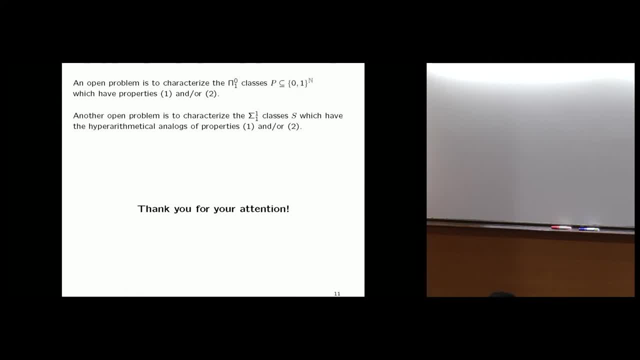 which have the hyper-arithmetical analogs of property one and two. We don't even know that there are any. we don't know that property one, property two holds in hyper-arithmetic theory. Forget about being belonging to the sigma one class. 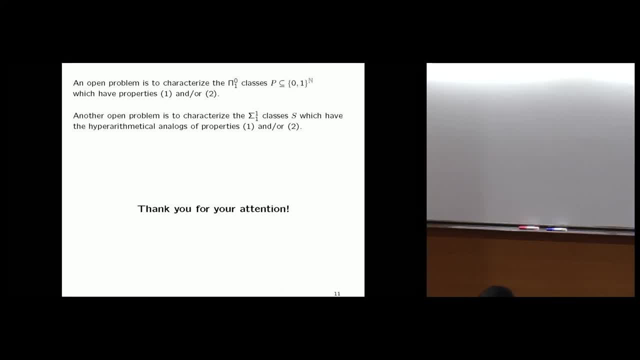 Another: these, these are just, you know, seem just seem like very natural questions that we've thought about, but we don't, we haven't made much progress on. So that's, that's. let me say that another. 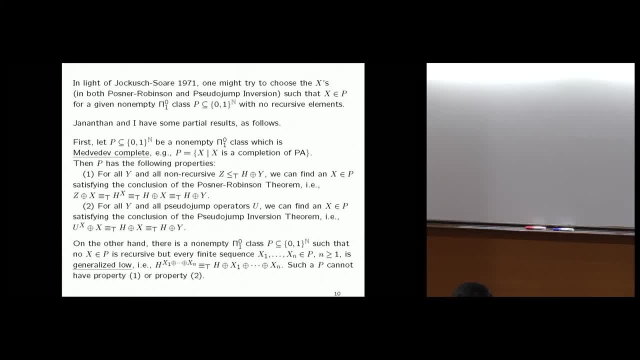 another subject that I'm very interested in is pi zero one classes and and their Muchnik degrees. They're, you know, viewing them as mass problems. I'm trying to write a book on this subject, but I'm you know it's going kind of slowly. 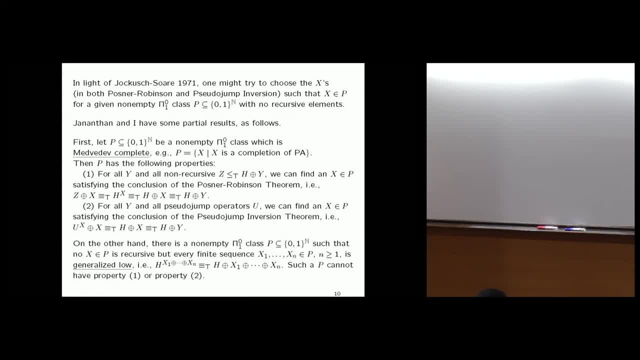 but I'll finish it, And so I was really. I'm really trying to get Jonathan to do that, but that subject, but we got sidetracked into this business in hyper-arithmetic theory. So that's about it. Thank you for your attention. 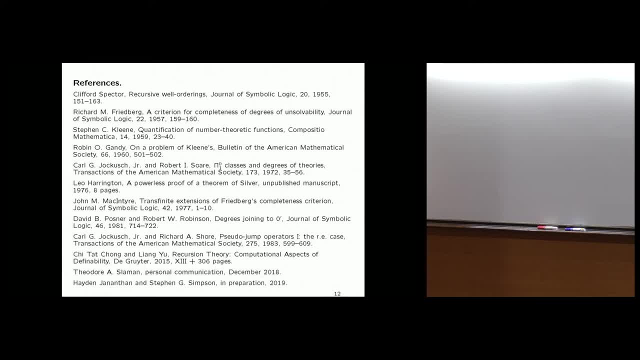 Here's the reference here this slide has. this slide has references to all the literature that I've cited here, Including the, the book by Chi-Tat Chang and Liang Yu, which you know is very appropriate here. Of course, they're both in the audience here. 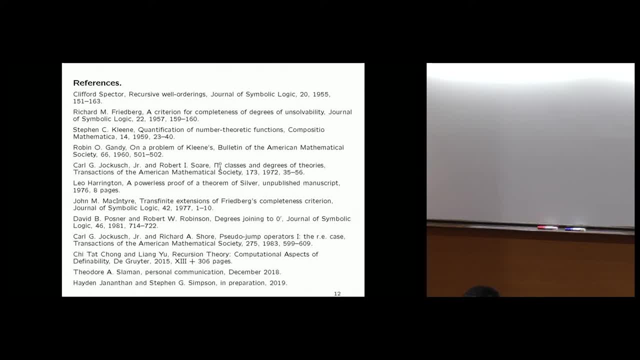 and Chi-Tat is the director of this whole thing, this institute, and so I was glad to be able to to cite their book And they they that that is an excellent modern reference for higher recursion theory. And let's see what else can I say about this? 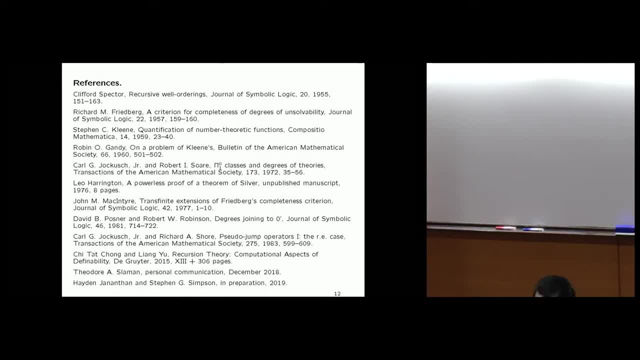 Yeah, okay, well, that's that's about it, Thank you Well, yeah, well, one of the obvious application. it's not really an application because its already known, but, for instance, there is a high degree less than zero prime. 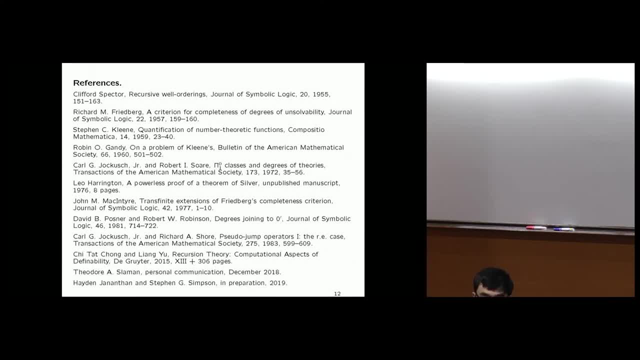 That. that just follows because As your pseudo-jump operator you take the construction of a low RE set, a low RE but non-recursive set. relativize that to X, that's a pseudo-hyperjump operation. Apply the pseudo-hyperjump inversion theorem with that operator to get a degree, to get: 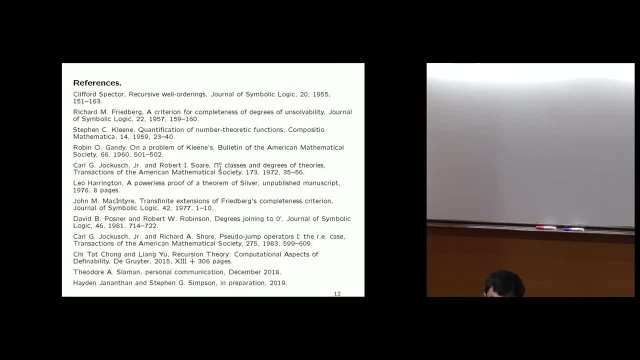 an X whose pseudo-jump- that is, a low RE set above it- is Turing equivalent to zero prime. Well then, the jump of that will be high. So you get for free a high degree less than zero prime. Now, that's the application we had in mind. 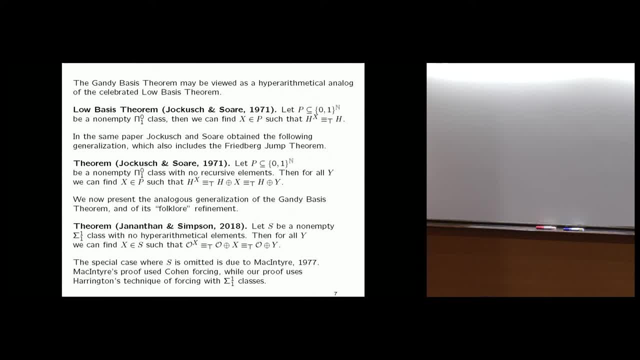 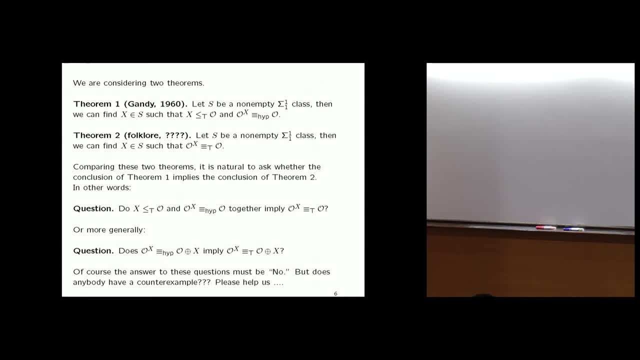 And you see this open question. the strategy we had in mind for proving this was to generalize the pseudo-hyperjump, you know, to prove the pseudo-hyperjump inversion theorem, which would give you, it wouldn't give you a high degree, it wouldn't give you the any kind. 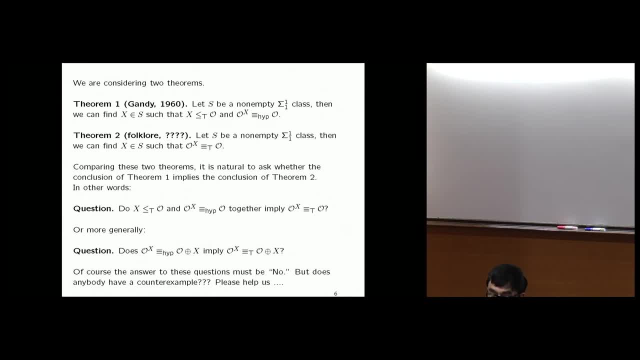 of analog of a high degree in hyper-arithmetic theory. but it would give you some, it would give you a counterexample to this thing. But we just weren't able to do that and we never thought of using sacks forcing. I should have thought of it myself. 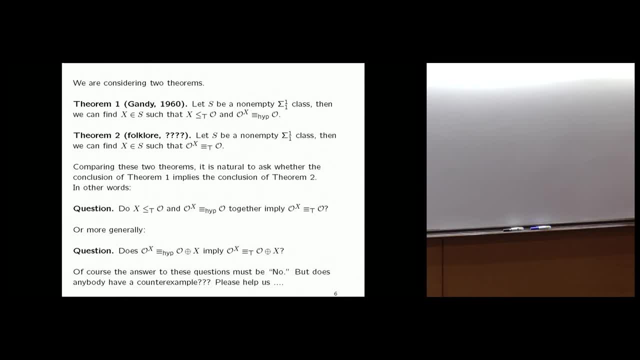 I mean, you know, I know all about that stuff, but Ted helped me, steered me the right way there. I mean, well, he gave me the answer to that question And gave us the answer to that question, So yeah, so that's the kind of thing. 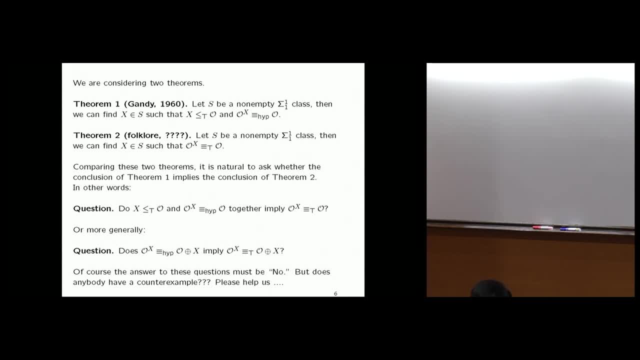 It's a powerful theorem They use. you know, Jockers and Shor use it to prove all kinds of things. You know, for instance, one problem. well, I had an old paper where I showed that. let's put it this way. 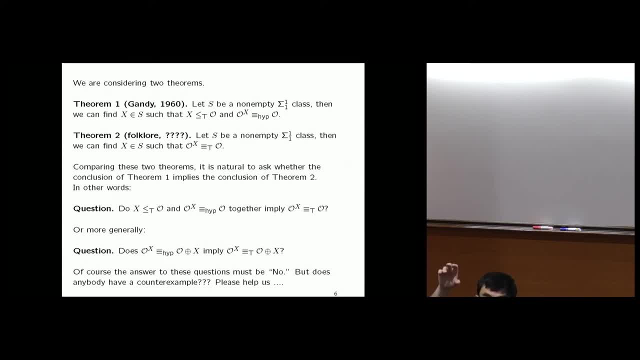 Zero sharp is the base of a cone of phi Of minimal covers in the hyperdegrees. all right, Zero sharp okay. And on the other hand, if V is a forcing extension of L, then there is no cone of minimal covers in the hyperdegrees. 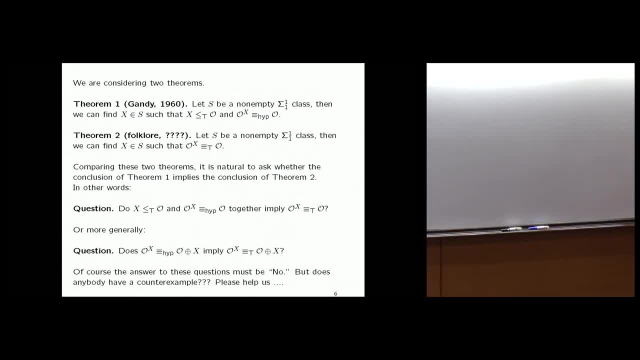 Now the Turing analog of that had been thought about and people wondered where is the base of the cone of minimal covers in the Turing degrees? And there's a paper where it was shown One that Kleene's O is the base of a cone for that. 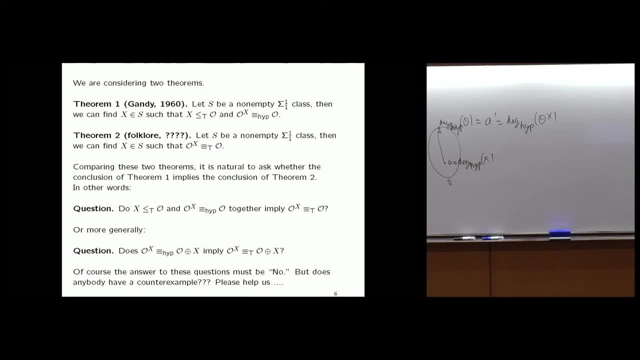 And Jockers and Shor use pseudo-hyperjump inversion, or some jazzed up version of it, to prove that zero to the omega, the arithmetical jump of zero, is the base of a cone. So that's- and they that's- just one application that they do. 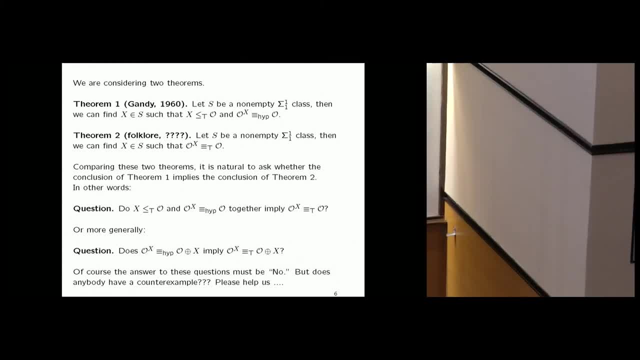 There's lots, lots of, lots of applications for that. So so, yeah, it seems very important and natural to do pseudo-hyperjump inversion, but we don't know how to do it. Okay, Yeah, well, there is no true analog of the PA degree.